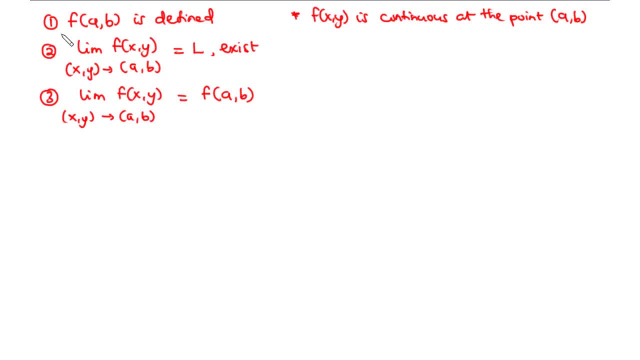 Now, in addition to that, even if only one of the conditions is being violated, then it means that the function cannot be continuous. Even if one of the conditions- either one, two or three- is violated, then it means that the function cannot be continuous at that. 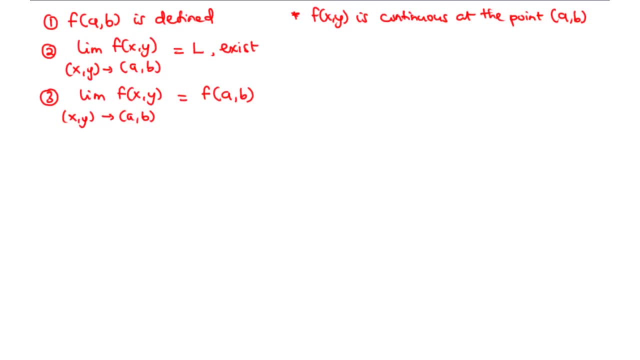 point. and if a function is continuous at every point in an open set d, then we say that the function is continuous on d. and then if a function is continuous at every point in the xy plane, then we say that the function is continuous everywhere. so let's try some examples. 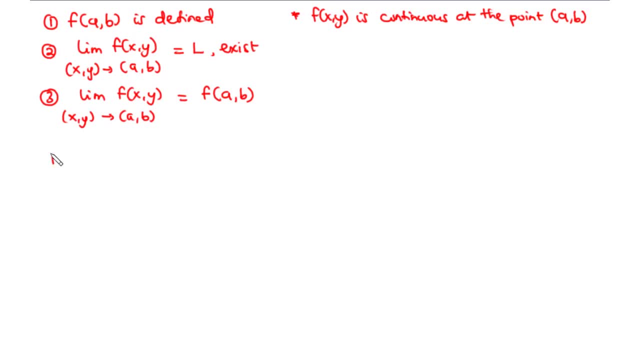 so giving two functions, f of x- y, that is 1. f of x- y is equal to 4 x square times y minus 3 x times y square, and then 2, we have g of x- y equals x square minus y square over x square plus y square. 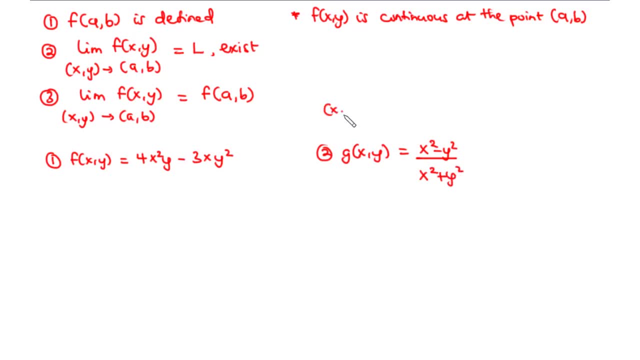 for all the functions that we have. and then we have a function f of x- y, that is 1, f of x- y is all the two functions we have, x- y- approaching the point zero zero prove whether or not the two functions are continuous at this point, at the point zero, zero. so let's try to solve. 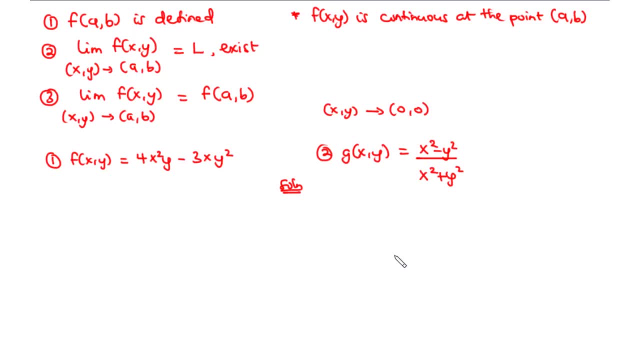 this example or these examples together. so for a function to be continuous at a set point, we say that f of a- b must be defined. secondly, the limit of the function. as x, y approaches a, b must exist, and then the limit of that function should be equal to the value of the function at the point a- b. so we are going to 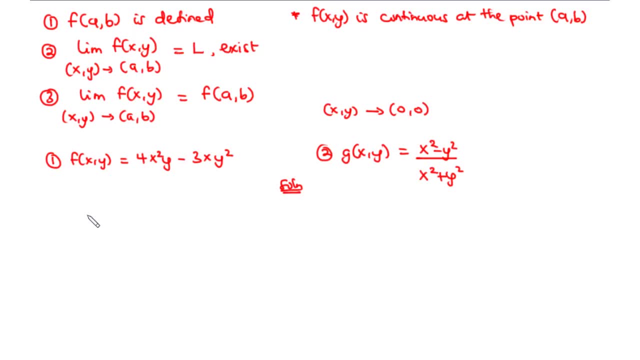 check for all these three conditions. so for the first question, we have f of x- y to be equal to 4 x square y minus 3 x y square. first we are going to look out for f of zero, zero and basically we are going to substitute. 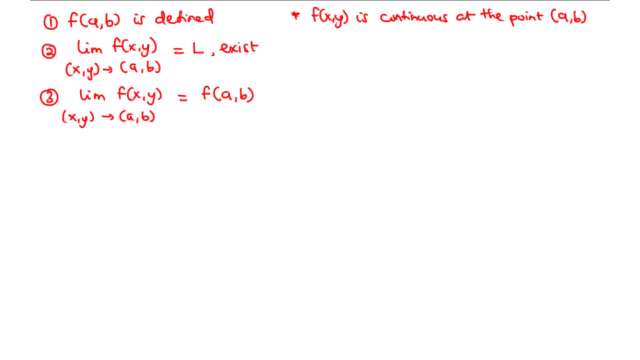 then we say that the function is continuous everywhere. So let's try some examples. So given two functions, f of x- y, that is 1, f of x- y is equal to 4x squared y minus 3x times y square. and then 2, we have g of x- y equals x square minus y. 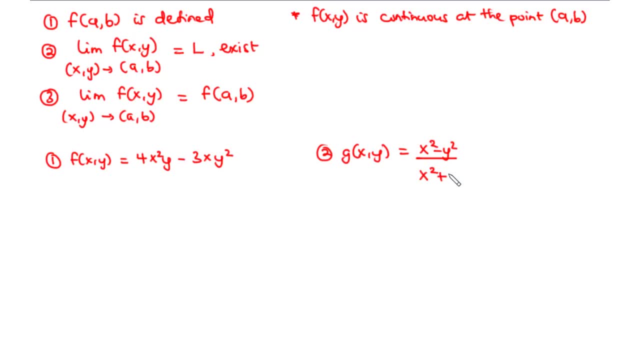 square over x square plus y square for all the two functions. we have x, y approaching the point 0: 0. prove whether or not the two functions are continuous at this point, at the point 0: 0. so let's try to solve this example or these: 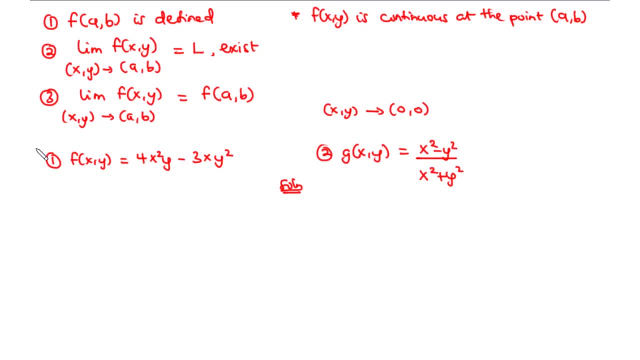 examples together. so for a function to be continuous at a set point, we say that f of a, B must be defined. secondly, the limit of the function. as X, Y approaches, a, B must exist, and then the limits of that function should be equal to the value of the. 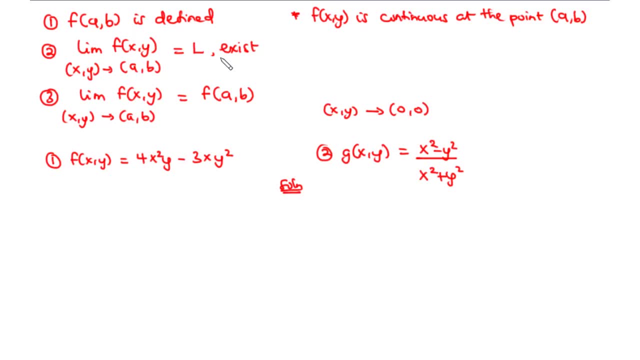 function at the point a, B. so we are going to check for all these three conditions. so for the first question, we have f of X- Y to be equal to 4x square Y minus 3 x y square. first we are going to look out for f of 0, 0 and basically 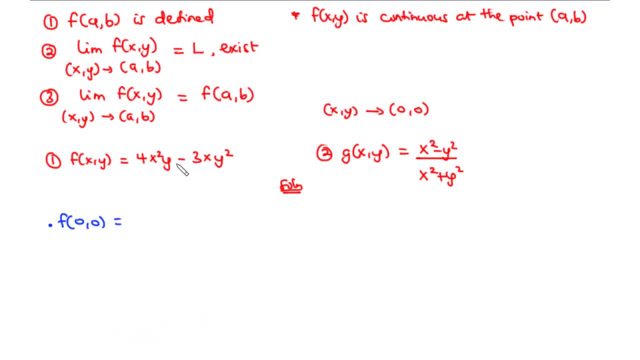 are going to substitute 0, 0 in place of X and then Y in this function, so we have 4 0 0 in place of X and then Y in this function. so we have 4 0 0 in place of X and then Y in this function, so we have 4. 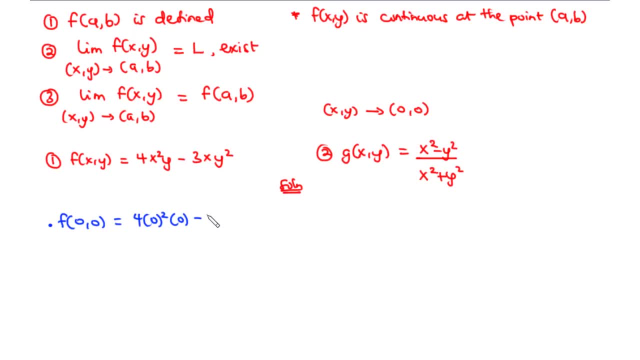 times 0 square, times 0 minus 3 times 0 times 0 square, and then 0 times 0 times 4 gives us 0 minus. this also goes to 0. so we have f of 0. 0 equals 0. now let's move on to the limit now with. 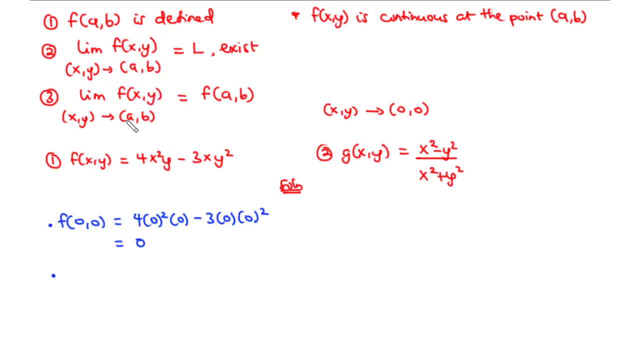 the limit we actually want to find or know how the function is going to behave as x- y approaches the point 0: 0, but not equal to 0: 0. so we take the limit of the function for x square y minus 3, x- y square as x- y approaches the point 0: 0. now, this is a polynomial function, so it supports: 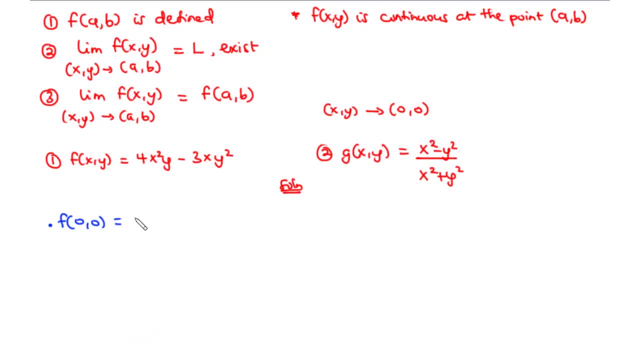 zero. zero in place of x and then y in this function. so we have four times zero square times zero minus. three times zero times zero square, and then zero times zero times four gives us zero minus. this also goes to zero. so we have f of zero. zero equals zero. now let's move on. 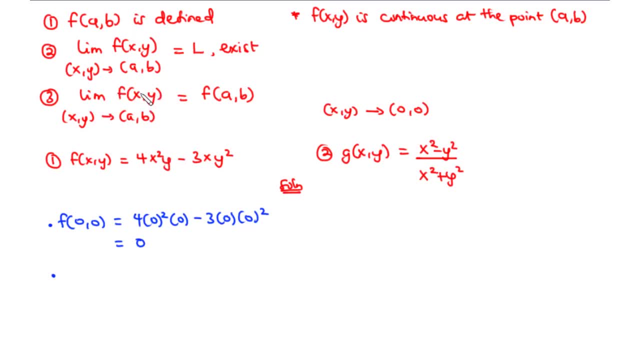 to the limit. now, with the limit, we actually want to find or know how the function is going to behave as x- y approaches the point zero zero, but not equal to zero zero. so we take the limit of the function for x square, y minus three, x- y square as x- y approaches the 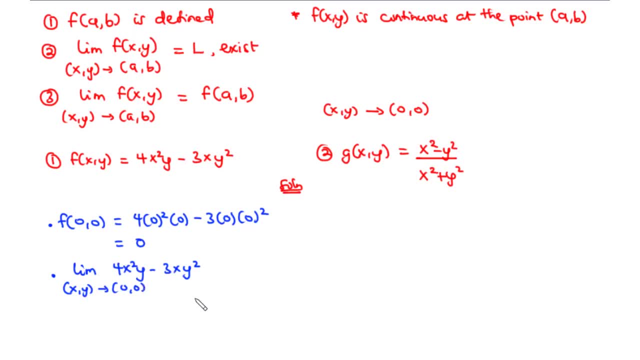 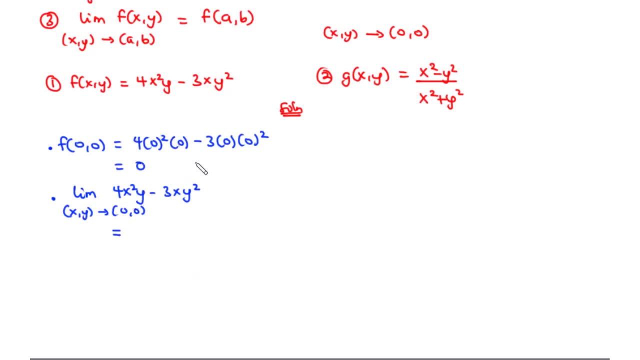 point zero, zero. now this is a polynomial function, so it supports direct substitution. so we are going to directly substitute in zero, zero in place of x and then y, as we here. So also we are going to have 4 times 0 square times 0 minus 3 times 0 times 0 square. 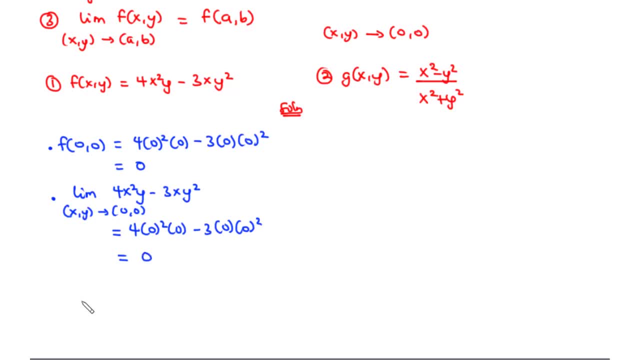 and actually we are going to have the same answer, which is 0.. Therefore, since the limits of the function f of x- y as x y approaches 0, 0 exist and is equal to the value of the function at the point 0, 0, that is, is equal to the point or is equal to f of 0, 0, we say that: 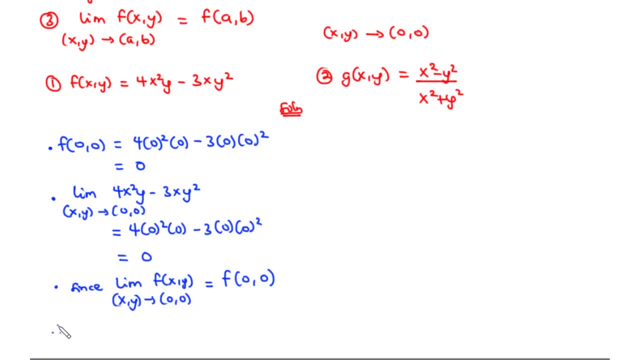 the function. therefore the function f of x- y is continuous, is continuous at the point 0: 0. the function is continuous at the point 0: 0. now again, because this is a polynomial function. then it means that a polynomial function is always continuous at every point in the x- y plane, because we have no restrictions on x and the y. 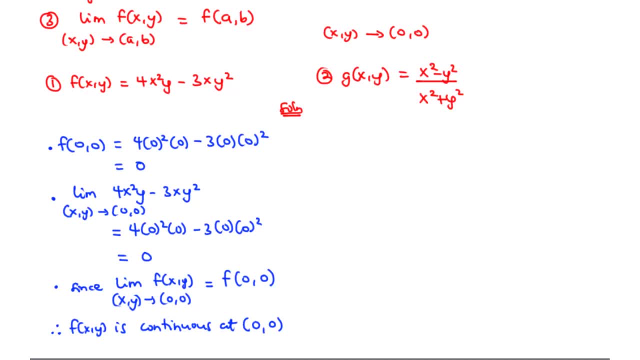 so since this is also a polynomial function, it means that this function is also continuous everywhere in the x y plane. so now let's move on to the second example. for the second example we have: g of x- y equals x square minus y square, divided by x square plus y. 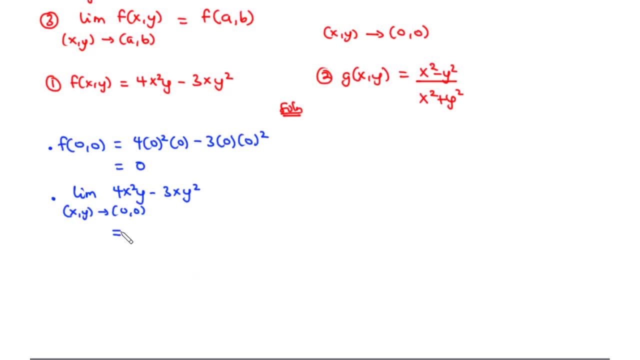 direct substitution. so we are going to directly substitute in 0: 0 in place of x and then y, as we did here. so also we are going to have 4 times 0 square times 0 minus 3 times 0 times 0 square and actually we are going to have the. 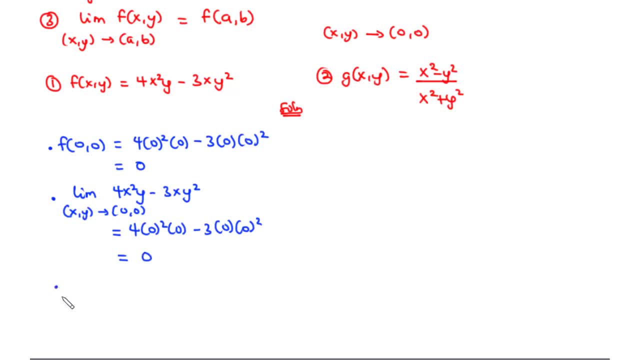 same answer, which is 0. therefore, since the limits of the function f of x- y as x y approaches, 0, 0 exists and is equal to the value of the function at the point 0, 0 and therefore we are going to have the same answer, which is 0, that is, is equal to the point or is equal to f of 0, 0. we say that the 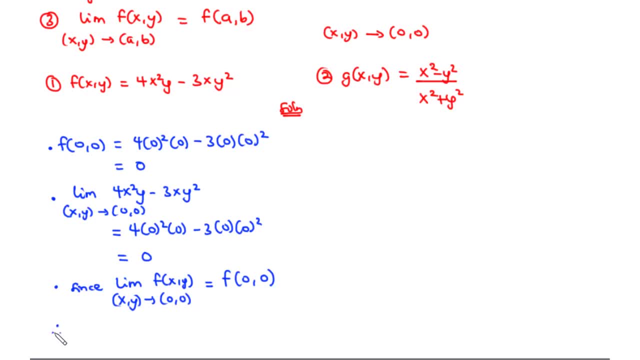 function. therefore the function f of x, y is continuous, is continuous at the point 0: 0. the function is continuous at the point 0: 0. now again, because this is a polynomial function. then it means that a polynomial function is always continuous at every point in. 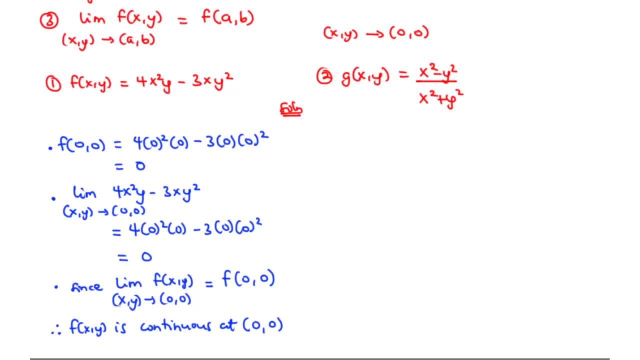 the x y plane because we have no restrictions on x and the y. so since this is also a polynomial function, it means that this function is also continuous everywhere in the x y plane. so now let's move on to the second example. for the second example we have: g of x. y equals x square minus y. 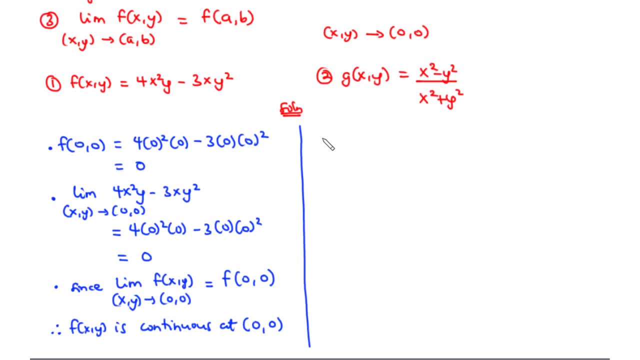 square divided by x square plus y square. so first of all, we are going to look out for g of 0: 0. you basically substitute 0: 0 in place of x and y. we have 0 square, 0 square minus 0 square all divided. 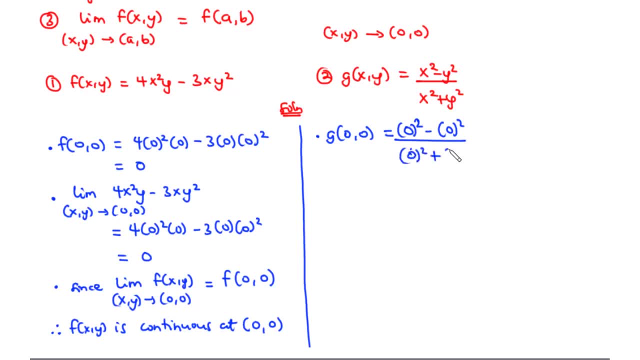 by 0 square plus 0 square, this is equal to 0 divided by 0, and this is indeterminate. this is indeterminate. indeterminate means we don't actually know what value this is going to be. i mean, we don't know what 0 over 0 is. so it's indeterminate now, since the value of the function is not defined at. 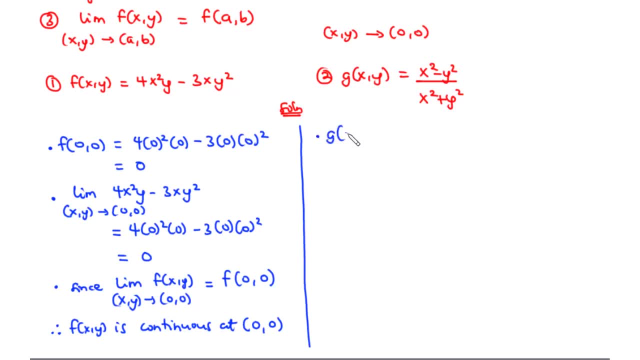 square. so, first of all, we are going to look out for g of 0: 0. you basically substitute 0: 0 in place of x and y. we have zero square, zero square minus zero square. all divided by zero square plus zero square, this is equal to zero divided by zero, and this is indeterminate. this is indeterminate. 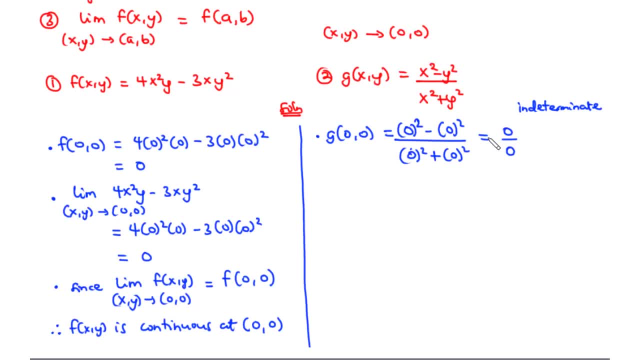 indeterminate means we don't actually know what value this is going to be. i mean, we don't know what zero over zero is. so it's indeterminate. now, since the value of the function is not defined at g of zero, zero straight away, we can conclude that this function is not continuous at the point zero. 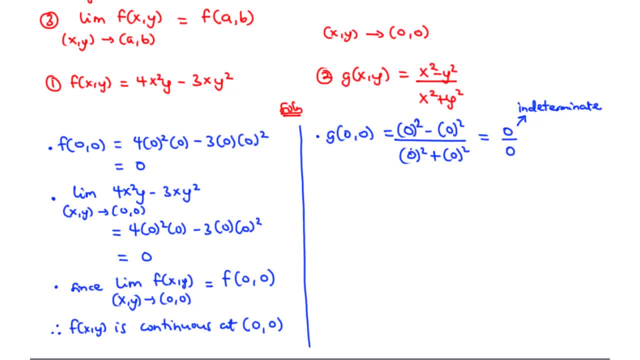 zero, because at least one of the conditions has been violated. now let's try to find the limit of this function, because it's going to be useful to us in the next example, even though the value of the limit is not going to change the fact that this function is not continuous at the point zero. 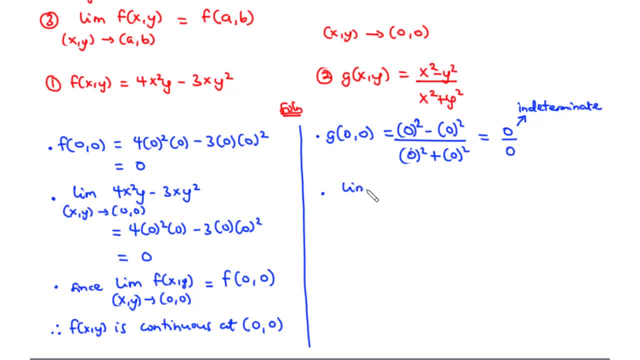 zero. so we try to find the limit of this function, that is, the limit of the function x square minus y square divided by x square plus y square, as x, y approaches the point zero, zero. so what we are going to do is we are going to approach, we are going to approach. 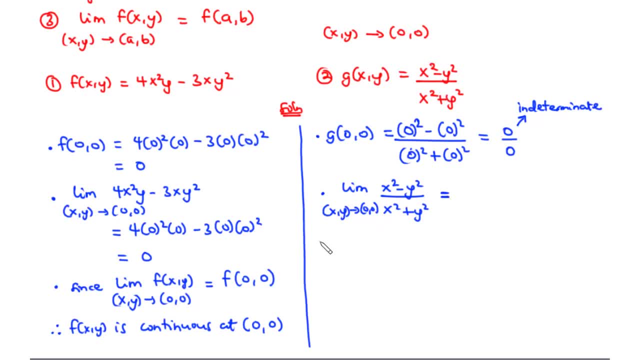 the point zero, zero from two different directions. so first of all we are going to approach, we approach the point zero, zero along the x-axis, along the x-axis, and then we know that along the x-axis, y is equal to zero. so we are going to put: y equals zero. so we have f of x, y that is equal. 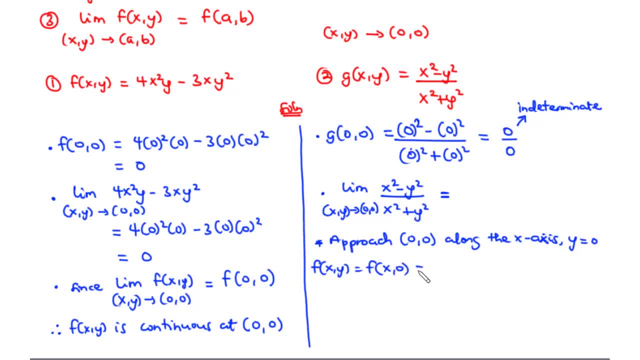 to f of x zero, and then we have the function. this becomes x square minus zero square divided by x square plus zero square, and this is going to be x square divided by x square, provided that x is not equal to zero, so this is equal to one. okay, so when we approach zero, zero along the x-axis, 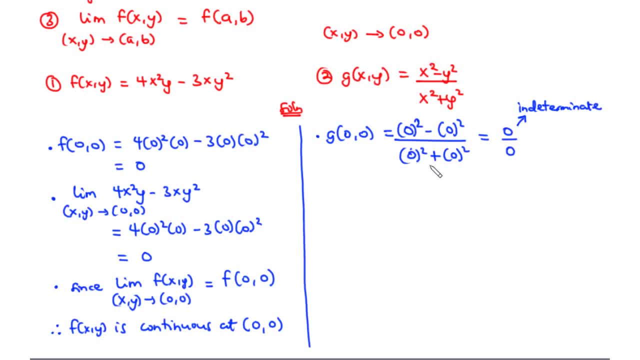 g of 0: 0. straight away, we can conclude that this function is not continuous at the point 0: 0, because at least one of the conditions has been violated. now let's try to find the lemma limit of this function, because it's going to be useful to us in the next example, even though the 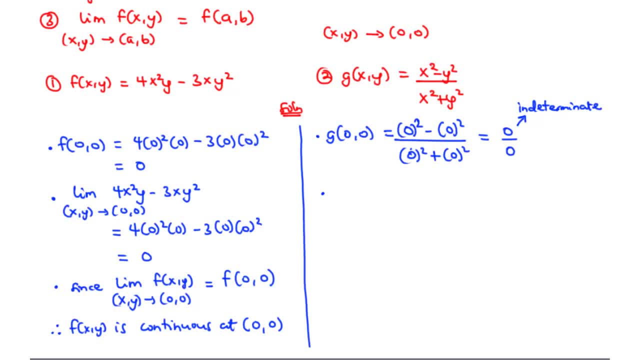 value of the limit is not going to change the fact that this function is not continuous at the point 0: 0. so we try to find the limit of this function. that is, the limit of the function x square minus y square divided by x square plus y square as x, y approaches the point 0: 0. so what we are going to? 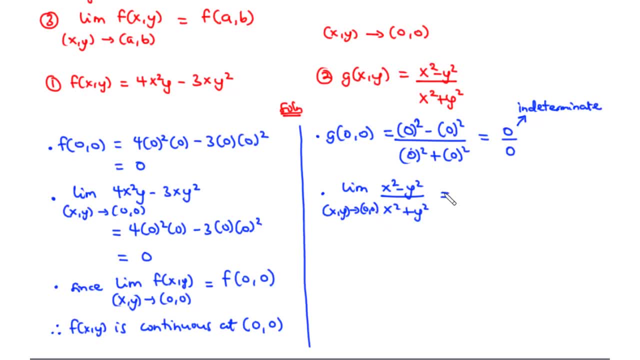 do is we are going to approach, we are going to approach the point zero, zero from two different directions. so, first of all, we are going to approach, we approach the point zero, zero along the x-axis, along the x-axis, and then we know that along the x-axis, y is equal to zero. 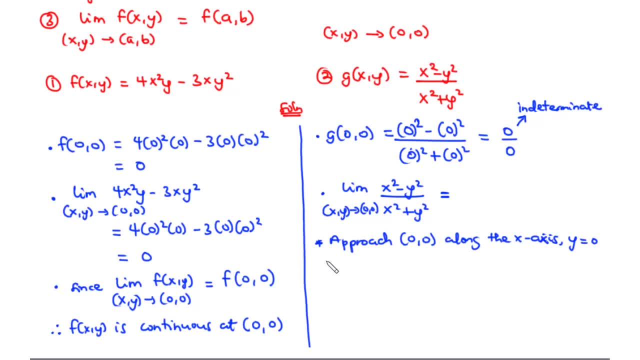 so we are going to put: y equals zero, so we have f of x- y that is equal to f of x- 0, and then we have the function. this becomes x square minus 0 square divided by x square plus 0 square, and this is going to be x square divided by x square, provided that x is not equal to. 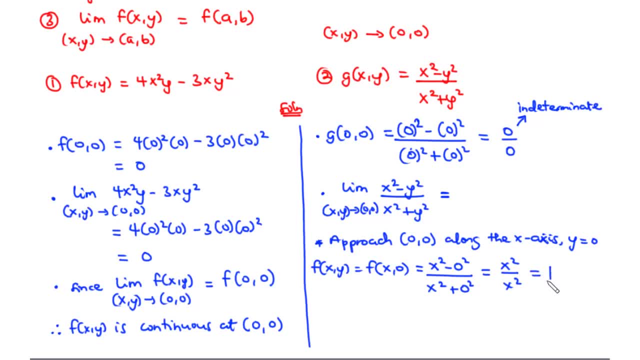 0.. so this is equal to 1. okay, so when we approach 0, 0 along the x-axis, we have this to be 1 again. let's approach, let's approach the point 0, 0 along the line, this time along the line, y equals x. so we have f of x, f of x, y equals. 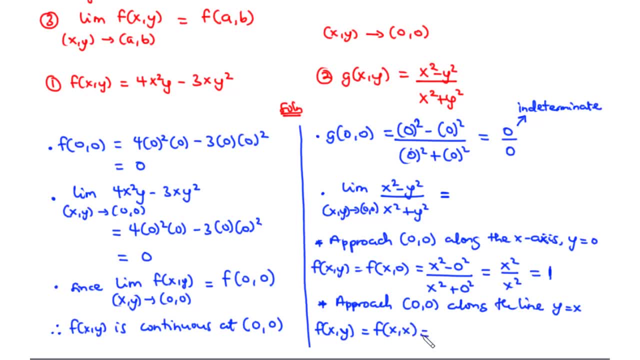 x. so we have f of x. y is equal to x, so however we see y, we are going to substitute x. so for this function, we have x square minus x square, divided by x square plus x square, and this is equal to 0 over 2 x square. and that is still 0. now, since we obtain: 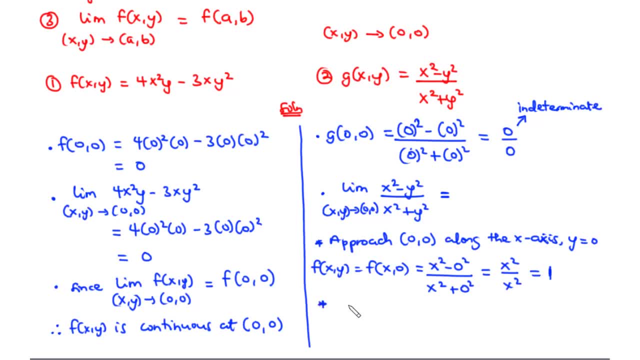 we have this function, and then we have the function: x square minus zero square divided by x square, by some, was to be one again. let's approach. let's approach the point zero. zero along the line, this time, along the line, y is equivalent to x. so, however we see y, we are going to substitute x. 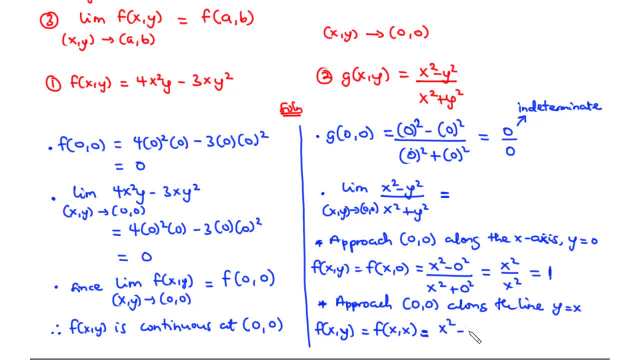 So for this function, we have x squared minus x squared, divided by x squared plus x squared, And this is equal to 0 over 2x squared, and that is still 0.. Now, since we obtained two different limit values for the two directions that we took, 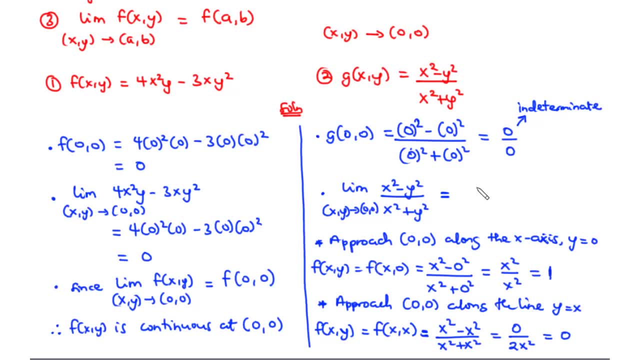 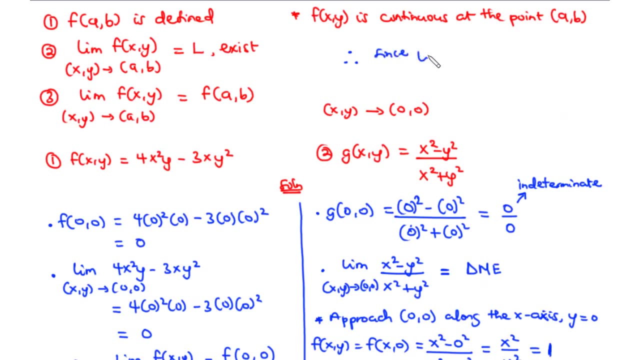 then it means that the limit of this function does not exist, because we have two different limit values for two different directions, So the limit of this function does not exist. Therefore, since the limit of the function g of x y, the limit of the function g of x y as x y approaches 0, 0, 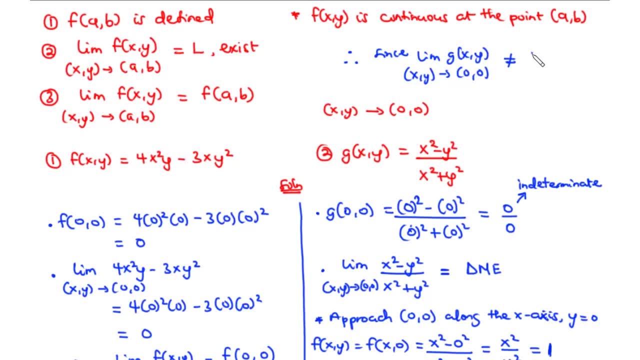 is not equal to the value of the function is not equal to the value of the function. at the point 0, 0, we say that g of x, y is not continuous. It's not continuous at the point 0, 0.. 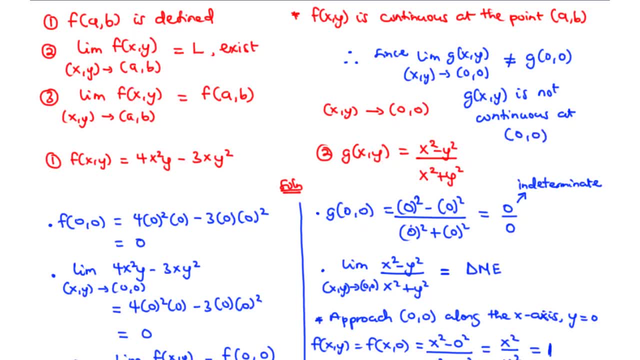 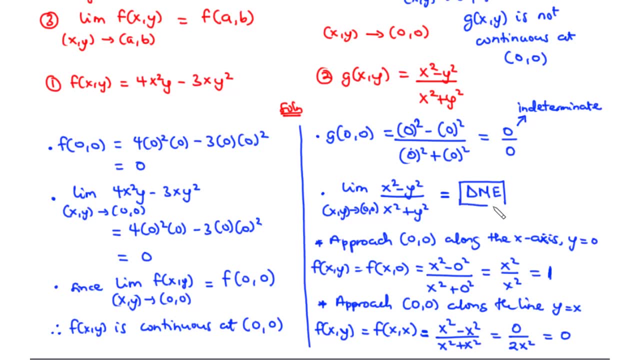 This function g of x- y is not continuous at the point 0, 0.. Now this is going to be useful to us in the next example. The limit of this function g of x- y is not continuous at the point 0, 0.. 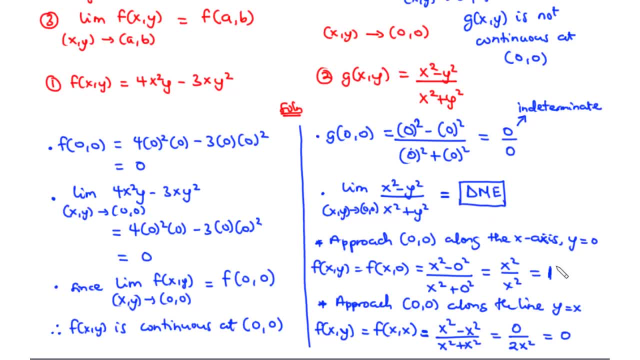 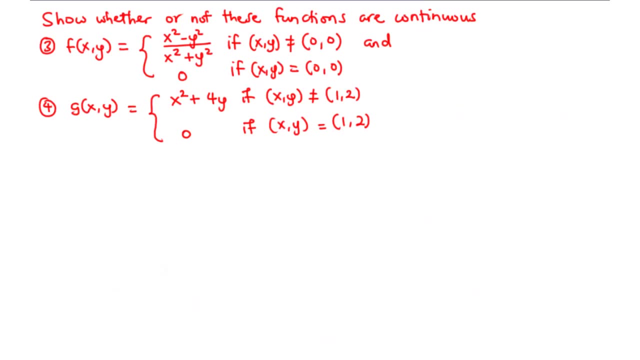 This function does not exist because we have two different limit values when we took two different directions approaching the point 0, 0.. Now let's move on as we take the next example. So for the next set of examples, we are going to consider some piecewise functions. 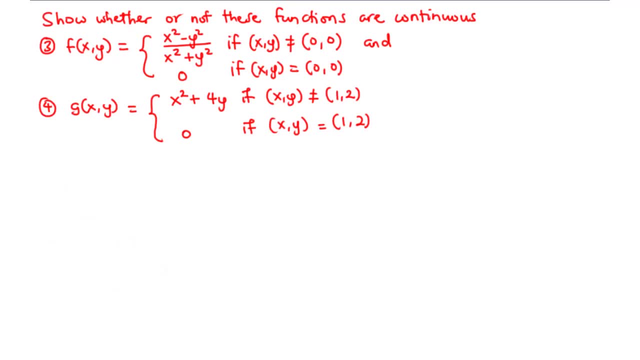 We are going to show whether or not these functions are continuous. So first of all let's start off with example 3.. So, for example 3, we have the function f of x. y equals x squared minus y squared over x squared plus y squared. 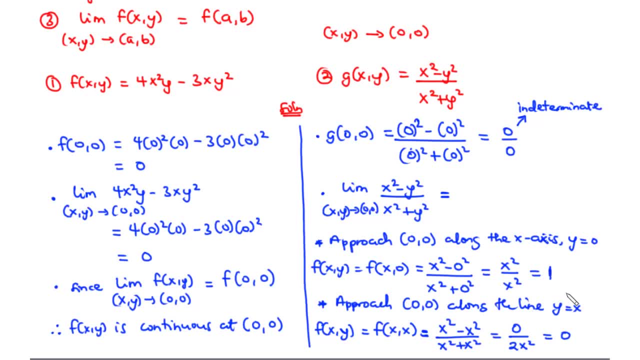 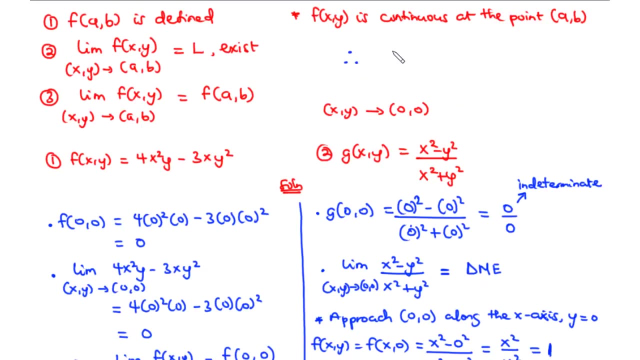 two different limit values. for that we took then it means that the limit of this function does not exist, because we have two different limit values for two different directions, so the limit of this function does not exist. therefore, since the limits of the function g of x, y, the limit of the function g. 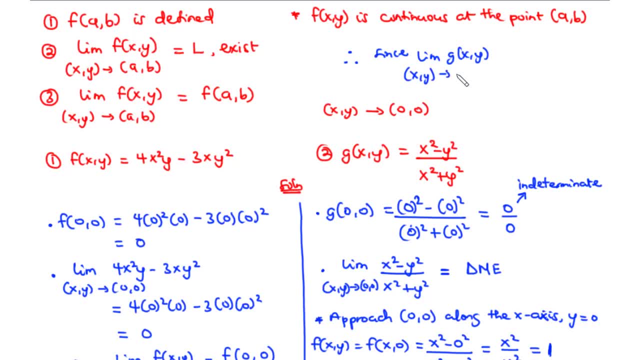 of x? y as x y approaches zero. zero is not equal to the value of the function, is not equal to the value of the function at the point zero zero. we say that g of x? y is not continuous. it's not continuous at the point zero zero. 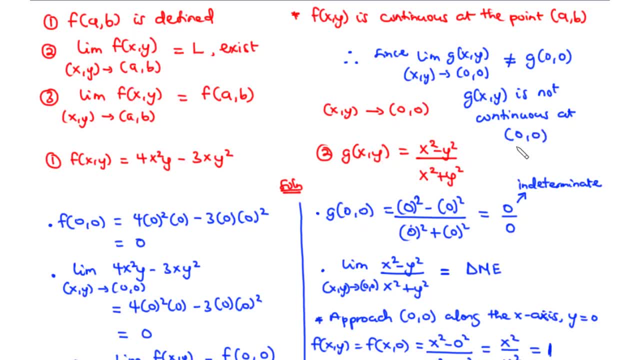 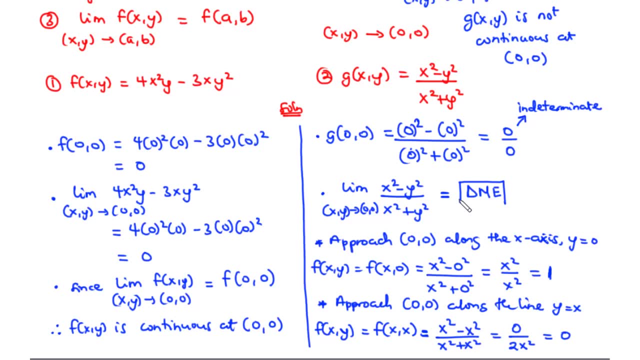 zero. this function g of x- y is not continuous at the point zero. zero now. this is going to be useful to us in the next example. the limit of this function does not exist because we have two different limit values when we took two different directions approaching the point zero. zero now. 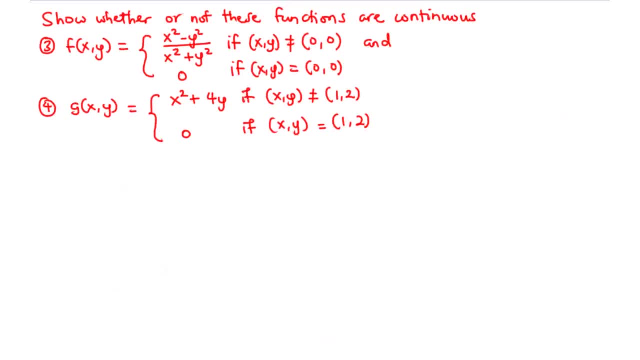 let's move on as we take the next example. so for the next set of examples, we are going to consider some piecewise functions. we are going to show whether or not these functions are continuous. so first of all, let's start off with example three. so, for example three, we have the function. 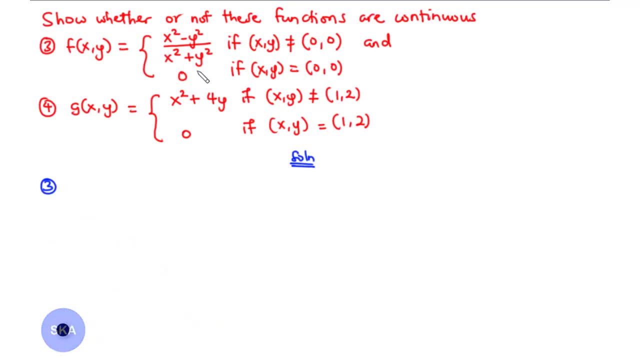 f of x- y equals x square minus y square over x square plus y square. if x- y is not equal to zero, zero and zero. if x- y is equal to zero, zero. now for this function to be continuous at the point zero, zero. first of all, we need to check if the function is continuous or not continuous. 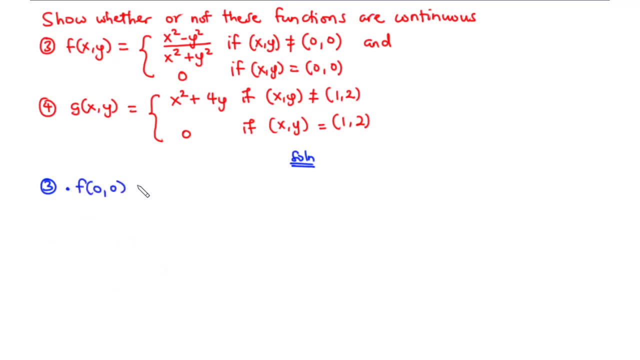 the first step is to define the limit of the function: n squared and c squared. so if we go back here and say x square minus y square plus plus y square plus c squared plus x square is continuous, then what we say is that x and y should always be continuous. 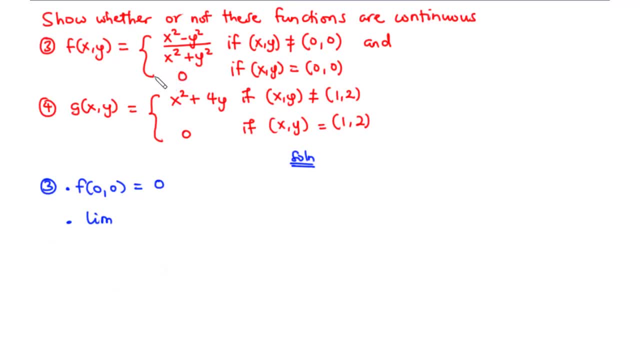 then it just superhero. we figure out that when x and y cross a relation, that the function is longitudinal from zero to x zero and we thought that that is the okay. this is what we mean by this. the value of the function is long, which means that 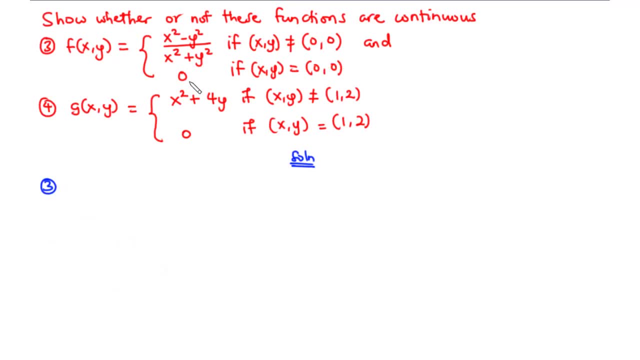 if x- y is not equal to 0, 0 and 0 if x- y is equal to 0, 0.. Now for this function to be continuous at the point 0, 0,. first of all, we need to check if the function is defined at the point 0, 0. 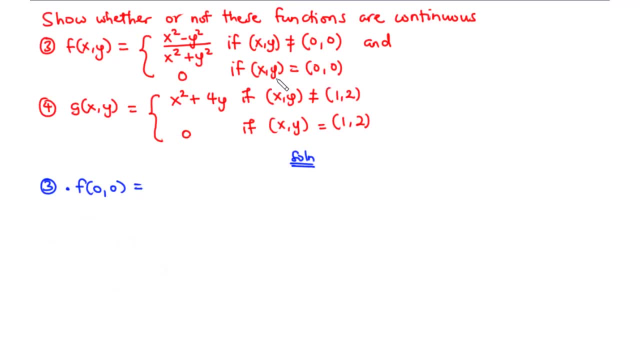 Now looking at the function, when x is equal to 0 and then y is equal to 0, we have the value of the function to be 0, which means that the function is defined at the point 0, 0.. 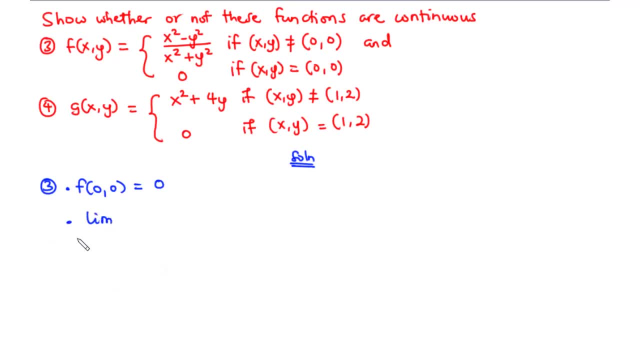 Now the next thing we are going to do is to find the limit of this function. So, as I said earlier in the previous example, we said that for the limit of a function, we basically want to know how the function is going to behave when you have x and then y approaching the point 0, 0. 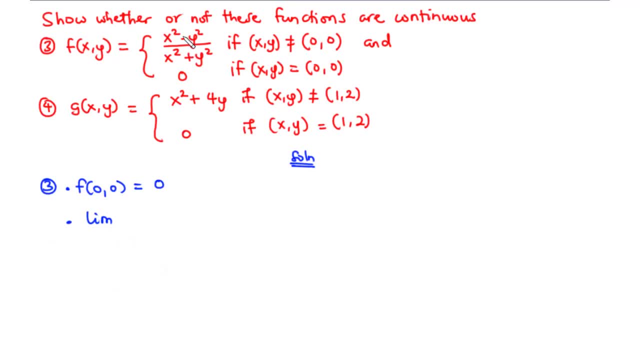 So we take the limit of this function, the limit of this function, which is x squared minus y squared over x squared plus y squared as x- y approaches 0. So we want to see how the function is going to behave when x- y approaches 0, 0 but not equal to 0.. 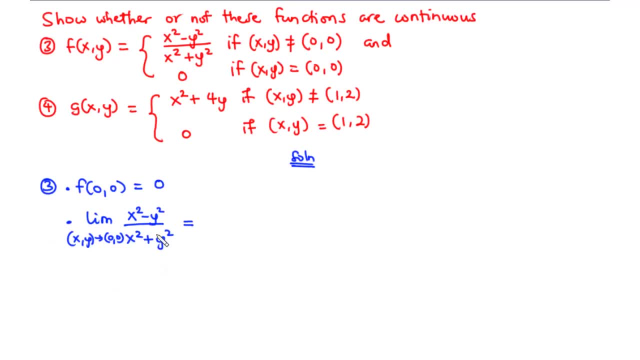 And then in example 2, you realize that the limit of this function did not exist. The limit of this function did not exist. Therefore, we say that since the limit of the function f of x y as x y approaches 0, 0,, 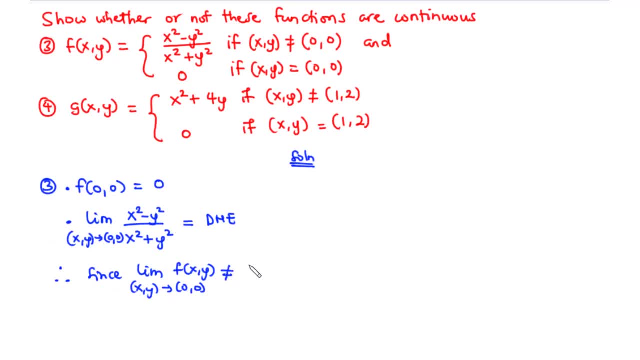 is not equal to the value of the function at the point 0, 0,. we say that the function f of x, y is not continuous. It's not continuous at the point 0, 0.. Let's try some more piecewise functions. 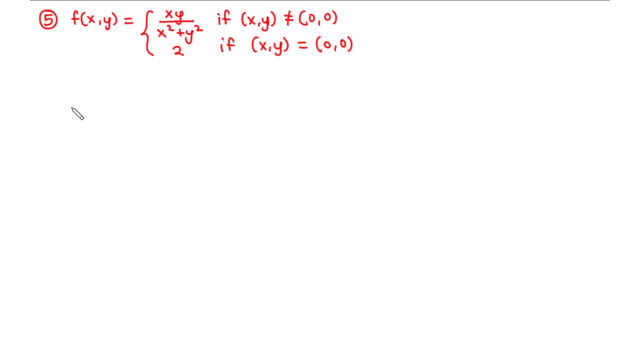 So here we have f of x y equals x y over x squared, plus y squared if x y is not equal to 0, 0, and then 2 if x y is equal to 0, 0.. Let's try this example as well. 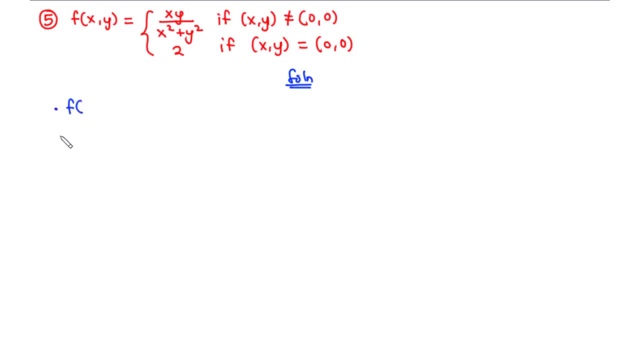 So first of all we are going to see if the value of the function at the point 0,, 0 is defined and that is equal to 2 from the question. So that is defined, f of 0, 0 is equal to 2.. 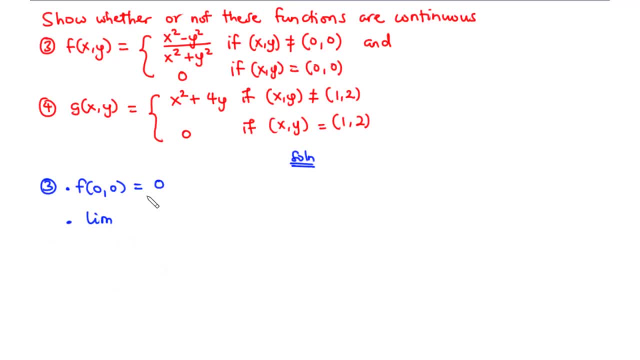 when x and y and y are continuous, it means that the function is continuous for the function area by approaching the point. So we take the limit of this function, the limit of this function, which is x square minus y square, over x square plus y square as x, y approaches. 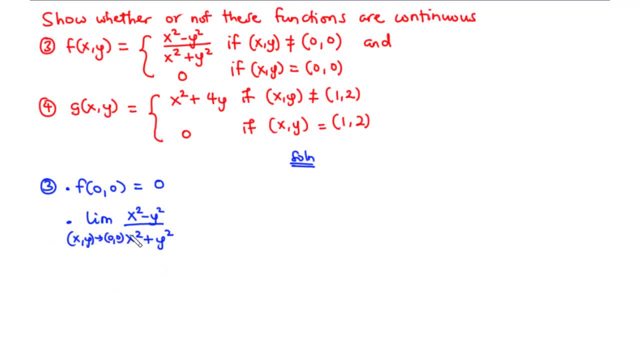 0. So we want to see how the function is going to behave when x, y approaches 0,, 0, but not equal to 0. And then in example 2, you realize that the limit of this function did not exist. the limit of this function did not exist. Therefore we say that since the limit of 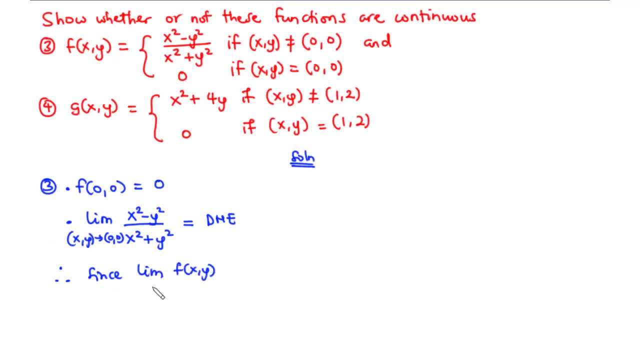 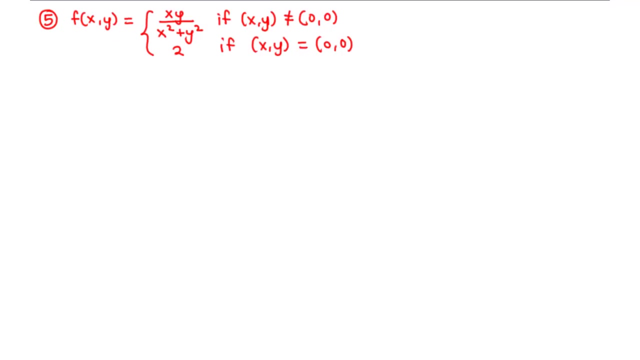 the function f as x, y approaches 0,. 0 is not equal to the value of the function at the point We say that the function f is not equal to the value of the function. not continuous. it's not continuous at the point: zero, zero. let's try some more piecewise functions. 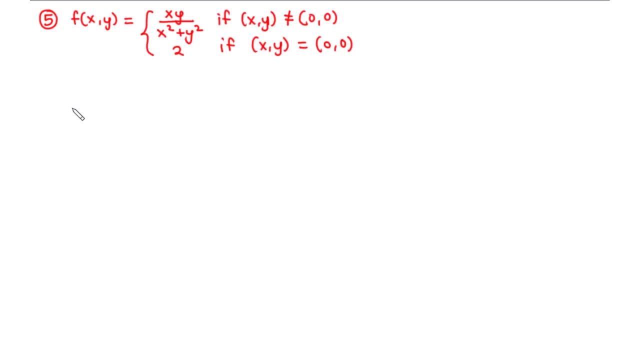 so here we have f of x- y equals x- y over x square, plus y square if x- y is not equal to zero zero. and then two: if x- y is equal to zero zero. let's try this example as well. so first of all, we are going to see if the value of the function at the point zero zero is defined, and that is: 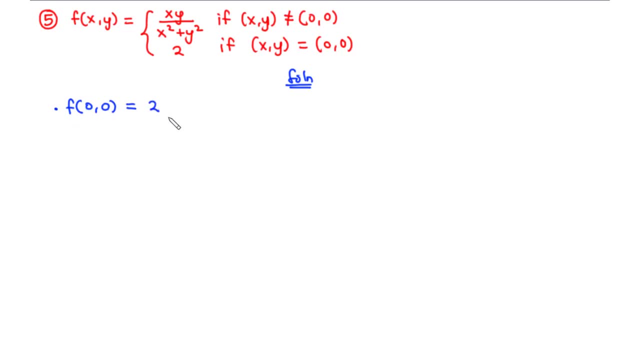 equal to two from the question. so that is defined. f of zero, zero is equal to two. the next thing is we want to find the limit of the function x times y divided by x square plus y square. as x, y approaches the point zero, zero, let's see if this function exists. 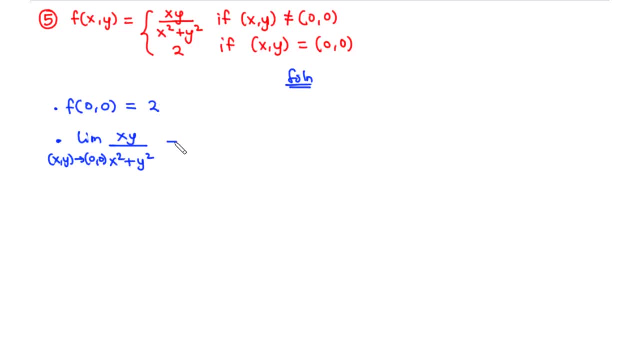 and is equal to two. so first, what we are going to do is we are going to approach the point zero, zero from two different directions. so first we want to, we want to approach, we want to approach the point zero, zero along the x-axis, along the x-axis, we know, along the x-axis, y is equal to zero. 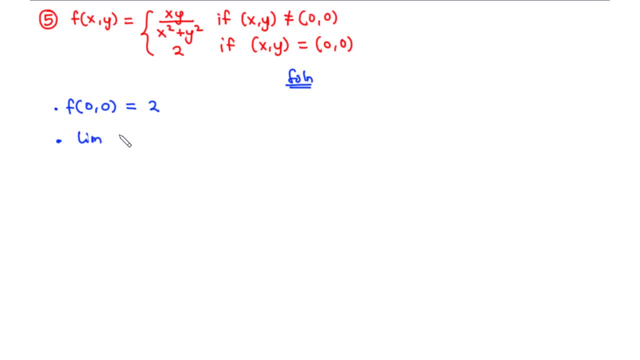 The next thing is we want to find the limit of the function x times y divided by x squared plus y squared as x, y approaches the point 0, 0.. Let's see if this function exists and is equal to 2.. 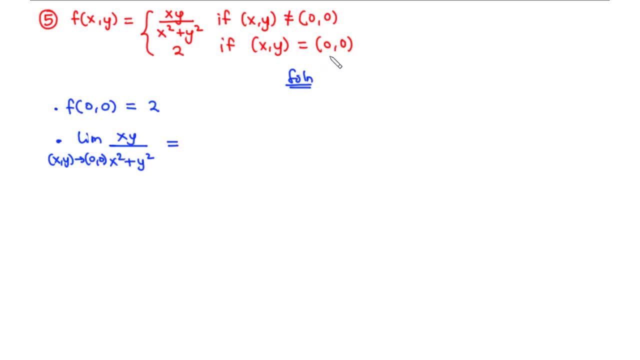 So first, what we are going to do is we are going to approach the point 0, 0 from two different directions. So first we want to approach. we want to approach the point 0, 0 along the x-axis. 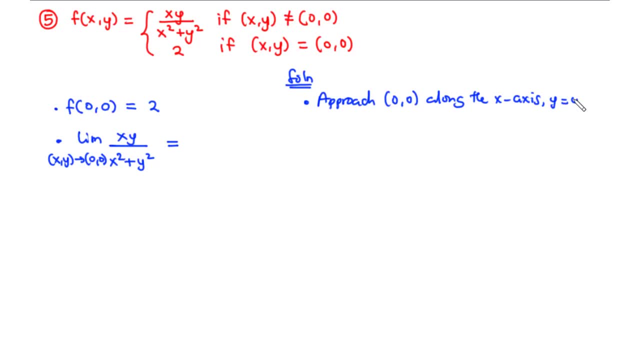 Along the x-axis. We know, along the x-axis, y is equal to 0. So we have f of x. y equals f of x- 0. Wherever we see y, we are going to substitute that for 0.. 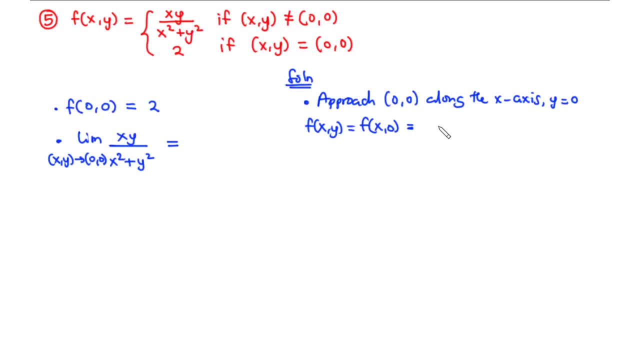 So we have for this function, we have x times 0, 0 over x squared, plus 0 squared, This is equal to 0 over x squared, provided x is not equal to 0. Then we say that this is equal to 0.. 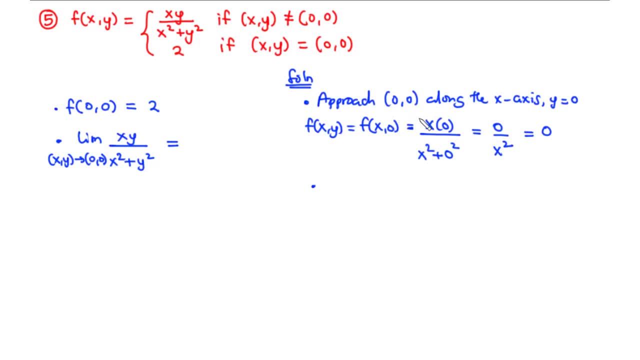 So this is the value we obtain after approaching the point 0, 0 along the x-axis. Now the next thing is: we are going to approach. we are going to approach the point 0, 0,, this time along the line. y is equal to x. 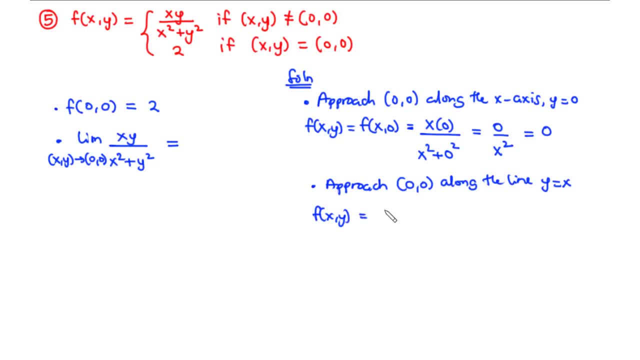 So here we have: f of x, y equals f of x, y is equal to x. So f of x- x, that is equal to x times x divided by x squared plus x squared, This is equal to x squared divided by 2x squared. 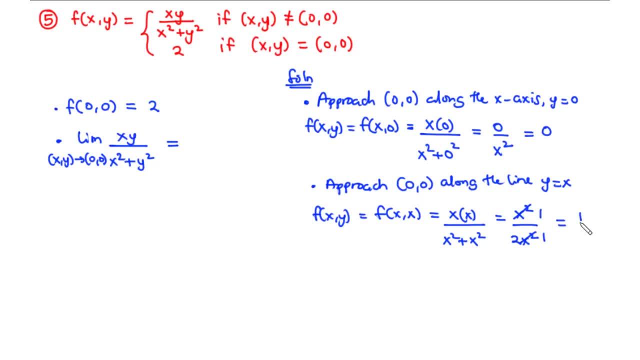 This goes here once. this goes here once. We are left with 0.. So we have f of x squared plus f of x squared, So f of x squared is equal to 1 over 2.. Now, since the two values are not the same, 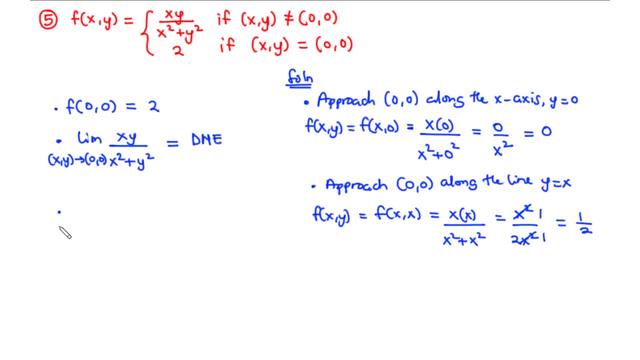 it means that the limits of this function does not exist. So the limits of this function, as x, y approaches 0, 0, does not exist. Therefore, since the limits of this function, that is, the limits of f, of x, y, 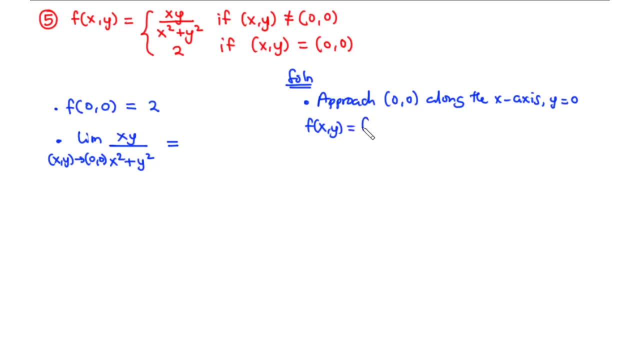 we have f of x. y equals f of x, zero. wherever we see y, we are going to substitute that's for zero. so we have for this function: we have x times zero over x square plus zero square. this is equal to zero over x square. provided x is not equal to zero, then we say that this is equal to zero. 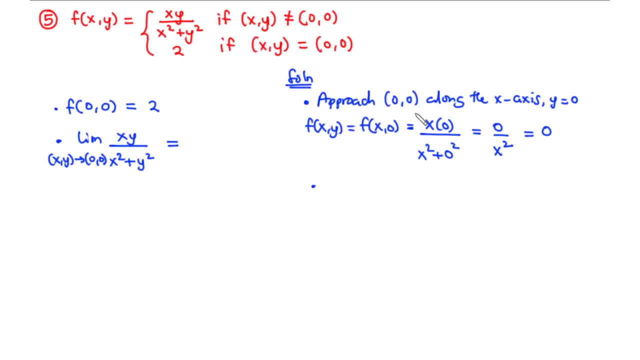 so this is the value we obtained out of this function. so we have f of x. y equals f of x- zero after approaching the point zero, zero along the x-axis. now the next thing is we are going to approach. we are going to approach the point zero, zero this time along the line y is equal to x. 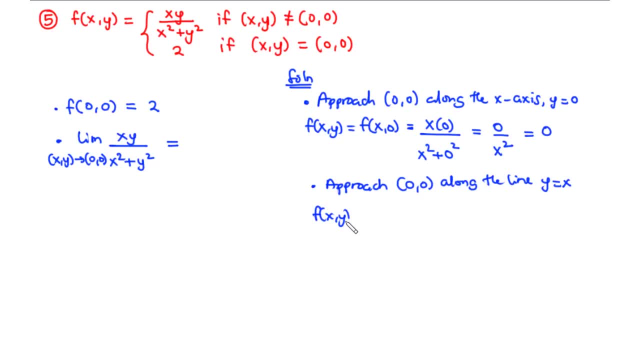 so here we have f of x. y equals f of x, y is equal to x. so f of x- x, that is equal to x times x divided by x square plus x square. this is equal to x square divided by two x square. this goes here once. this goes here once we are left with one over two. now, since the two values are not the same it. 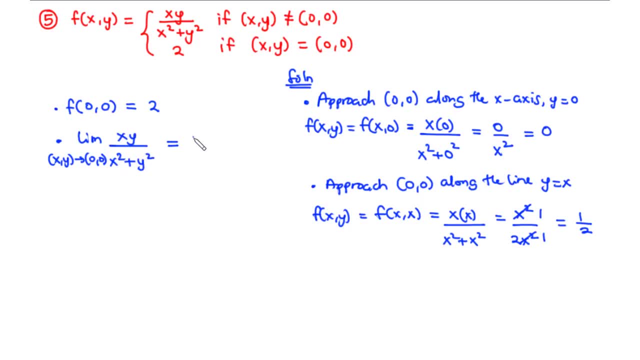 means that the limit of this function does not exist. so the limits of this function as x y approaches zero, zero does not exist. therefore, since the limits of this function, that is, the limit of f, of x- y, where we have x- y approaching the point zero, zero is not equal to the value of the function. 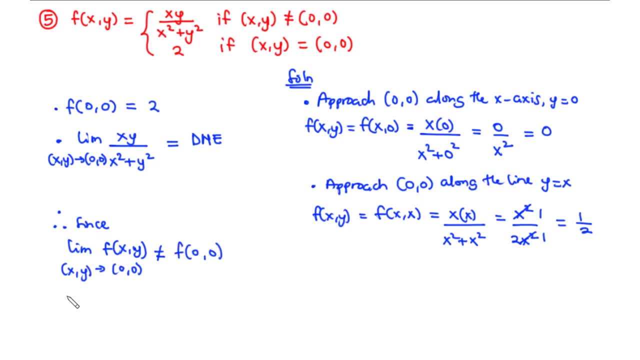 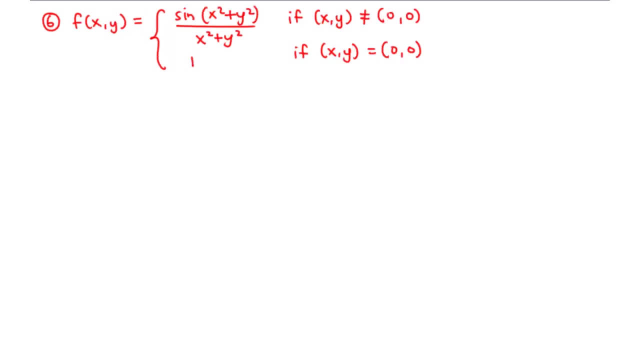 at zero, zero. we say that the function, the function f of x, y is not, it's not continuous at the point zero, zero. now let's move on to the next example. so, for example six, we have f of x, y equals sine into bracket x square plus y square over. 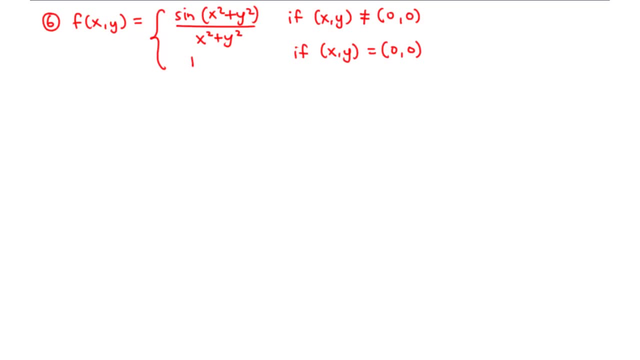 x square plus y square. if x- y is not equal to zero zero, and then one if x- y is equal to zero zero. let's solve this as well. so, first of all, we have f of zero zero, giving us one in the question. so so the value of the 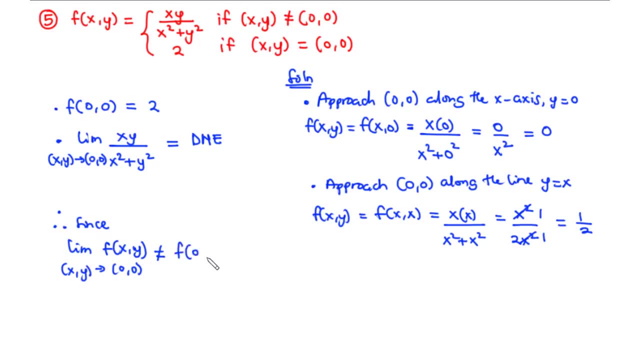 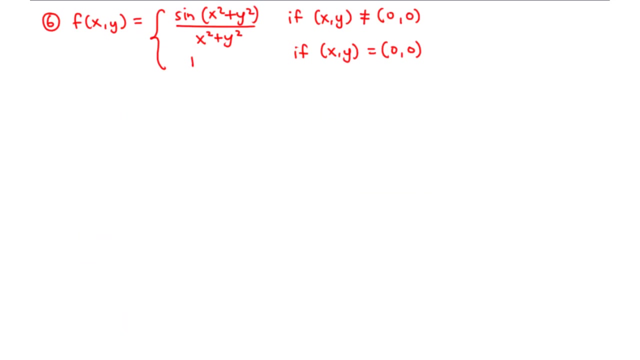 is not equal to the value of the function at 0, 0.. We say that the function f of x- y is not continuous at the point 0, 0.. Now let's move on to the next example. So for example 6, we have f of x- y equals sine into bracket x squared plus y squared over, x squared plus y squared, if x- y is not equal to 0, 0.. 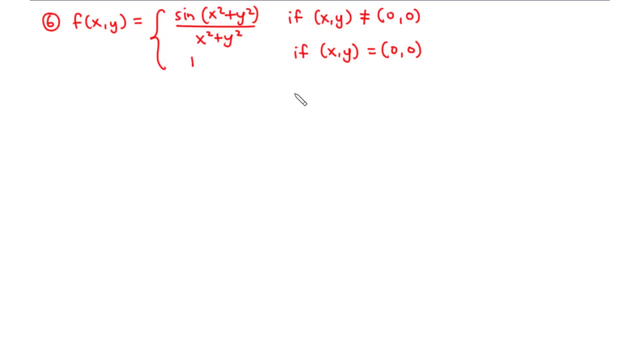 And then 1 if x, y is equal to 0, 0.. Let's solve this as well. So first of all, we have f of 0, 0, giving us 1 in the question. So the value of the function is different. 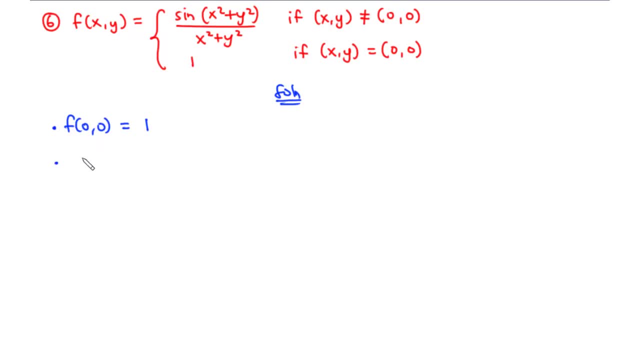 We find at the point 0, 0, and that is equal to 1.. Next thing, we want to find the limits of this function, So the limits of the function sine x squared plus y squared, all divided by x squared plus y squared, as x, y approaches the point 0, 0.. 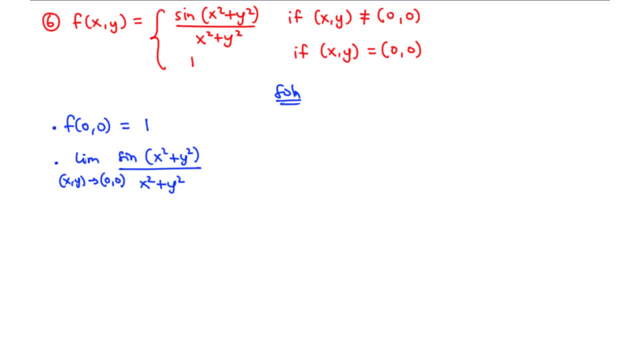 Now, in this example, we are going to use what we call the polar coordinate approach. So how do we solve that using the polar coordinate approach? So what we are going to do is we are going to let r and then theta be the polar coordinates of x, y. 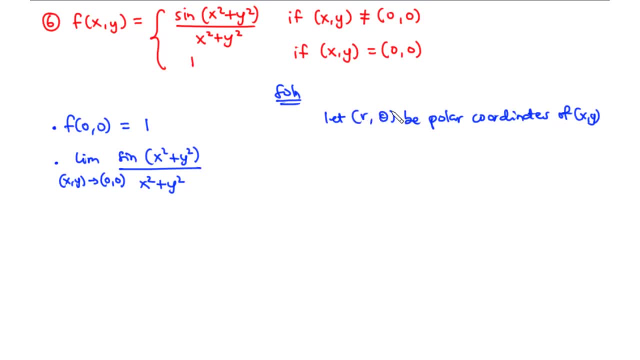 Now r here is called the modulus, and then theta here is called the argument from complex numbers. So what we are going to do here is we know that r squared is equal to x squared plus y squared, And then we are going to take r to be greater than or equal to 0.. 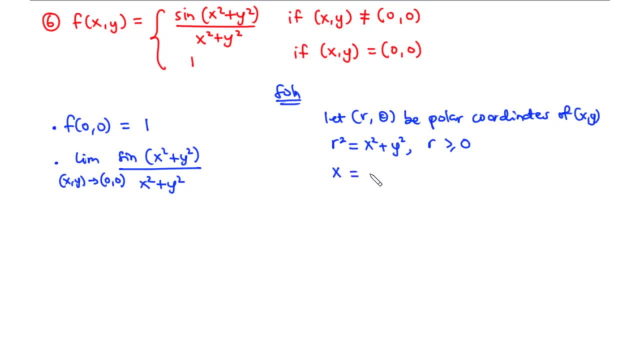 So from algebra we know that x is equal to r cos theta, And then we have y to be r sine theta. So basically, we are going to substitute either r squared Or x or y, depending on what we have as the function. 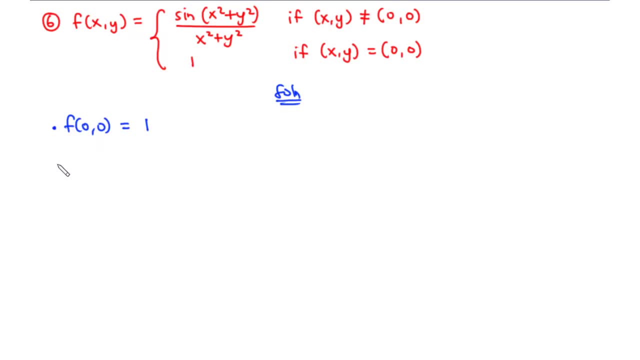 function is defined at the point zero, zero, and that is equal to one. next thing: we want to find the limits of this function. so the limit of the function sine x square plus y square, all divided by x square plus y square, as x, y approaches zero, zero. so this is the limit of the function. 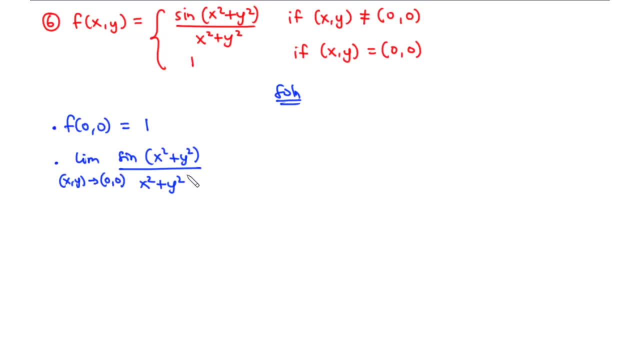 that is equal to x. x is equal to zero. zero won't be equal to 0, but this came out as going to be equal to 0, which is their point: zero, zero. now, in this example, we are going to use what you call the polar coordinates approach. so how do we solve that? 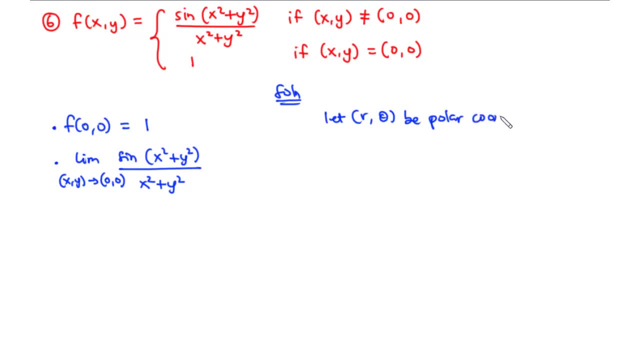 using the polar coordinates approach. so all we are going to do is we are going to let ourvity to be polar coordinates be the polar coordinates of R as a method. everybody here one over, and we have to be given the term it and let us x, y. now. r here is called the modulus and then theta here is called the argument. 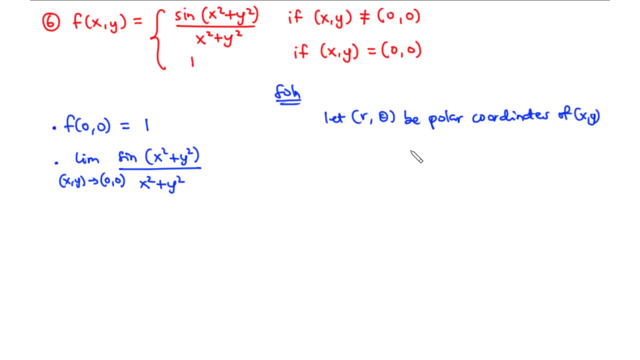 from complex numbers. so what we are going to do here is we know that r square is equal to x square plus y square, and then we are going to take r to be greater than or equal to zero. so from algebra we know that x is equal to r cos theta, and then we have y to be r sine theta. 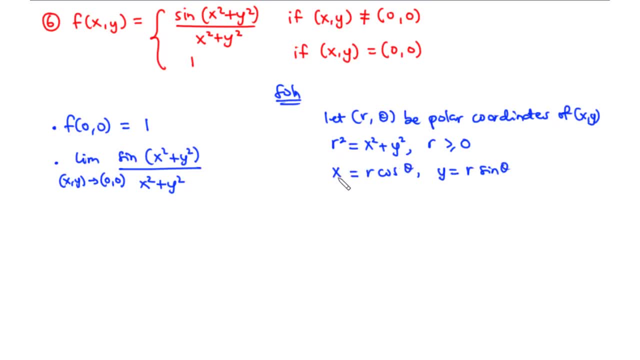 so basically, we are going to substitute either r square x or y, depending on what we have as the function. so let's continue to find the limit of this function. so here we have the limit of the function sine x square plus y square all over x square plus. 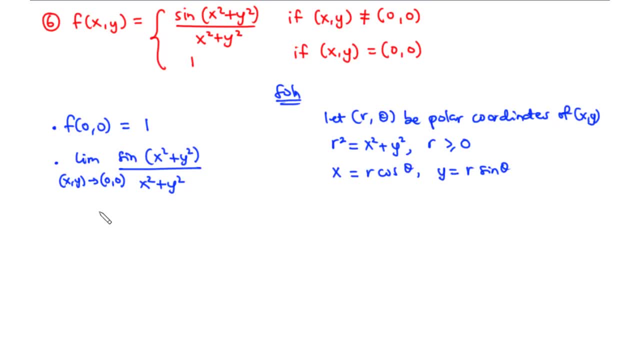 y square. now what we are going to do here is we are going to do direct substitution. so here we have the limit of the function. sine x square plus y square is equal to r square, so r square all divided by r square. and then, here for this, for this formula, as x and then y approaches. 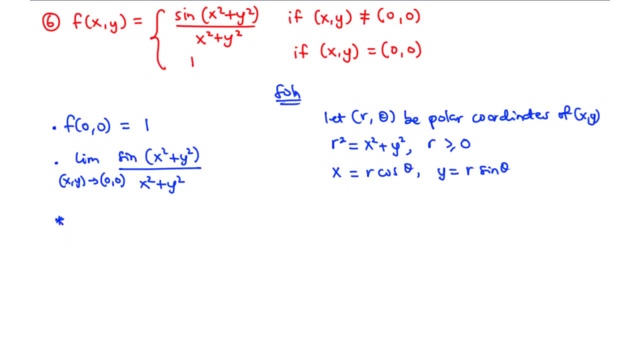 So let's continue to find the limits of this function. So here we have the limits of the function sine: x squared plus y squared, all over x squared plus y squared. Now what we are going to do here is we are going to do direct substitution. 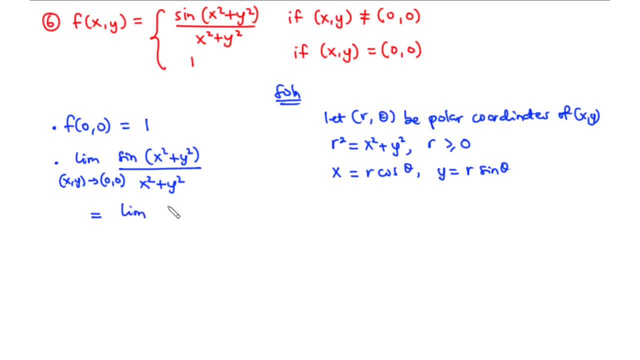 So here we have the limits of the function sine: x squared plus y squared is equal to r, So r squared all divided by r squared. And then here for this formula, as x and then y approaches 0, r also approaches 0.. 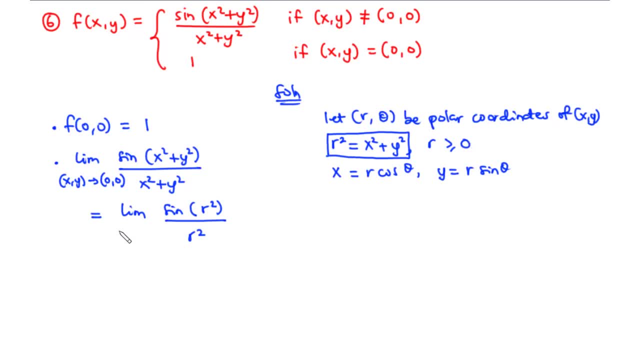 And then, since r is greater than or equal to 0, it means that r we are going to approach 0 from the right hand side. So Let's substitute 0 in place of r. So here we are going to have something like sine 0 over 0.. 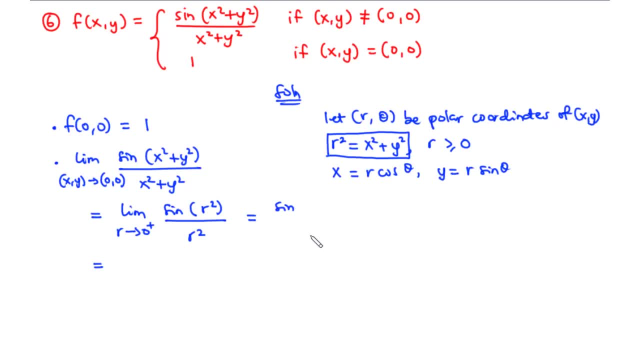 And sine 0 is 0. So 0 over 0 is indeterminate. Now, the moment we have after substituting the value of what the limit is approaching And then obtaining 0, 0, which is indeterminate, Then it brings the idea of using the L'Hopital's rule. 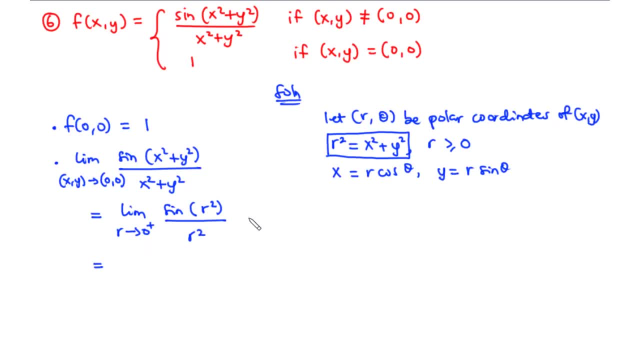 So we can use the L'Hopital's rule here, That is Given by The limit. So first of all let me have the formula here. So let's say, you have the limit of a function, So the limit, The limit of a function, f of x. 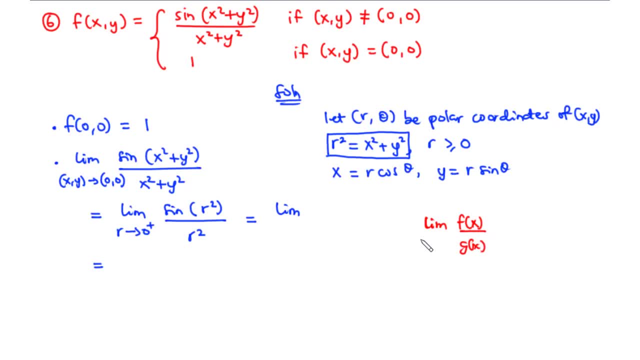 Divided by g of x As x approaches, let's say, 0.. Then, using the L'Hopital's rule, We say that this is equal to the limit of the first derivative of The function f of x divided by the first derivative of g of x as x approaches 0. 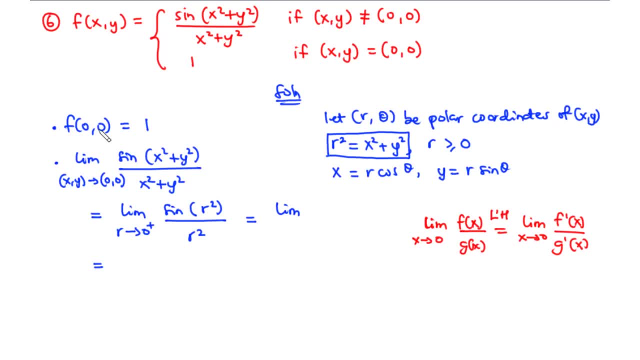 So basically, this is the idea we are going to use here. So here we have, using the L'Hopital's rule, We are going to have the limit of. Now let's try to differentiate this with respect to r. So when you differentiate what we have in the brackets, here we are going to have 2r. 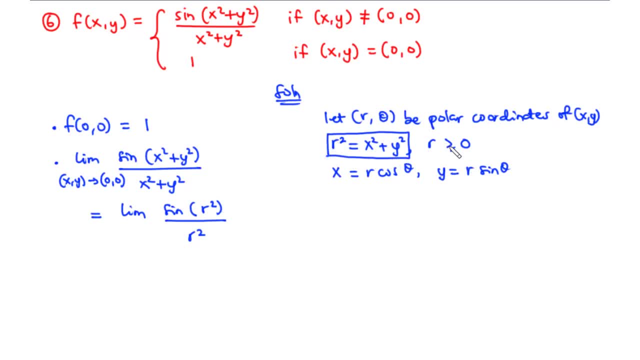 zero. r also approaches zero, and then, since r is greater than or equal to zero, it means that r, we are going to approach zero from the right hand side. so let's substitute zero in place of r. so here we are going to have something like sine zero over zero, and sine zero is zero. so zero over zero is indeterminate now, the moment we have. 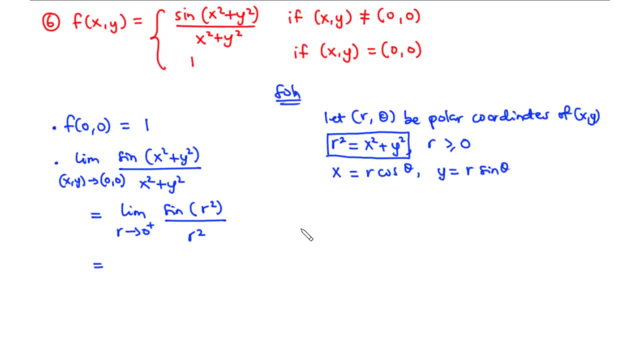 after substituting the value of what the limit is approaching and then obtaining zero, zero which is indeterminate. then it brings the idea of using the L'Hopital's rule. so we can use the L'Hopital's rule here that is given by the limit. so first of all let me have the formula here. so let's say you have 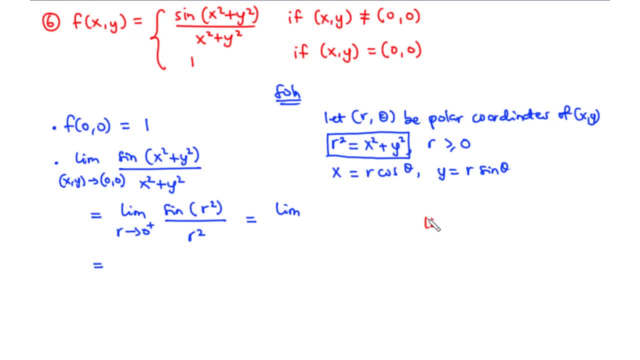 the limit of a function. so the limit, the limit of a function, f of x divided by g of x. as x approaches, let's say, zero, then using the L'Hopital's rule, we say that this is equal to the limit of the first derivative of. 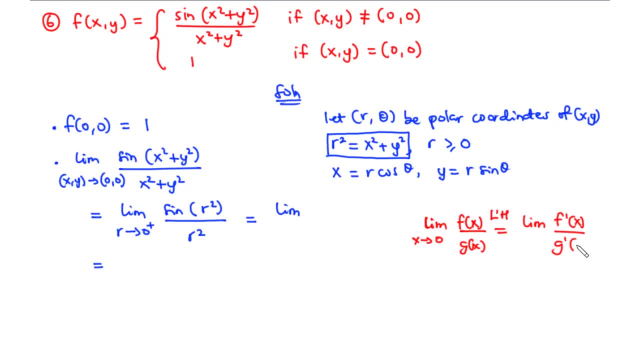 the function f of x divided by the first derivative of g of x, as x approaches zero. so basically, this is the idea we are going to use here. so here we have, using the L'Hopital's rule, we are going to have the limit of. now let's try to differentiate this with respect to r. 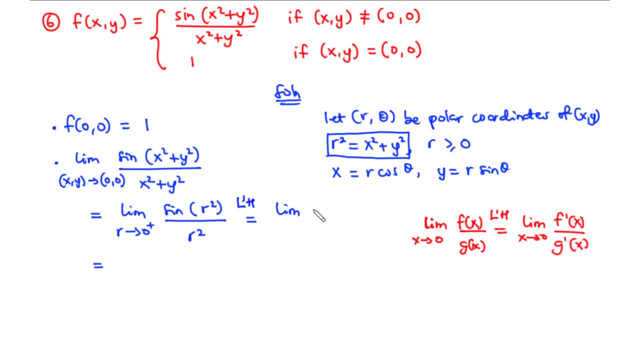 so when you differentiate what we have in the brackets here, we are going to have two r, and then when you differentiate sine, you have cos and then you repeat r squared divided by for the bottom function, we are going to have two r as r approaches zero. 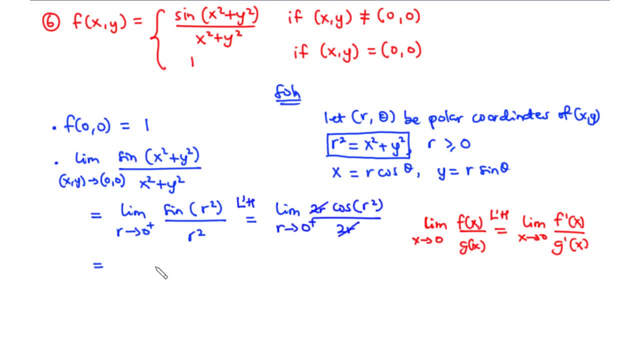 from the right. so 2r cancels out 2r and then we are left with cos r squared. we do direct substitution of 0 and then we have cos 0 squared, which is equal to 0, so cos 0 and then cos 0 is. 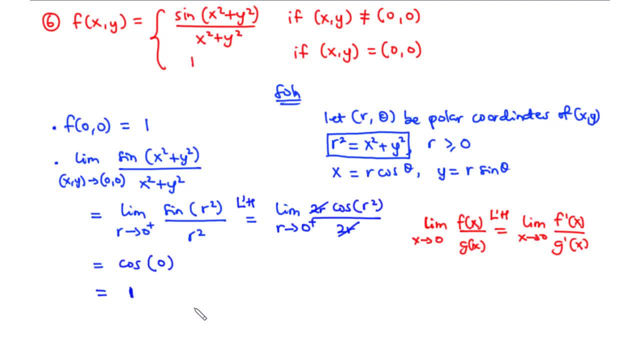 equal to 1. now notice that whenever your last expression depends on theta, it depends on theta. it means that the limit of the function does not exist. and again, even if you obtain a real value for the limit of the function, it does not necessarily mean that the limit of the function 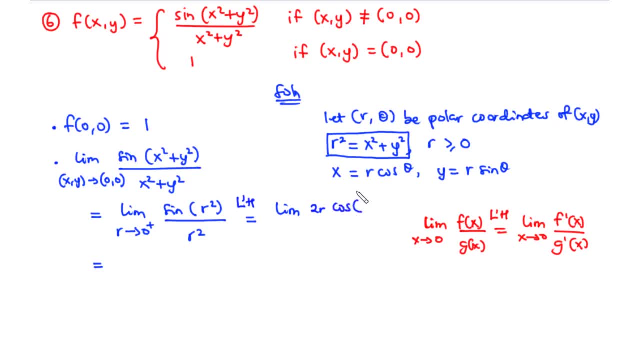 And then when you differentiate sine, you have cos And then you repeat r squared Divided by. For the bottom function, we are going to have 2r As r approaches 0 from the right. So 2r cancels out 2r. 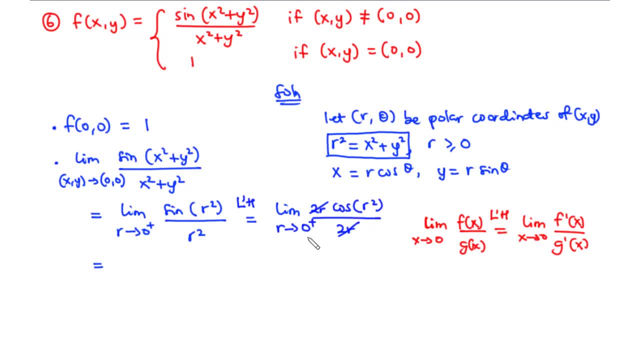 And then we are left with cos r squared. We do direct substitution of 0. And then we have cos 0 squared, Which is equal to 0.. So cos 0. And then cos 0 is equal to 1.. Now notice that whenever your last expression 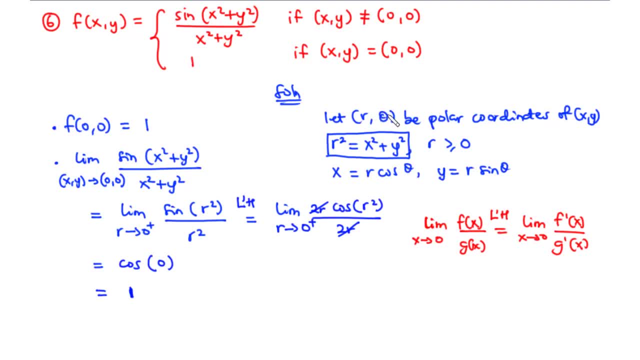 Depends on theta. It depends on theta. It means that the limit of the function does not exist. And again, even if you obtain a real value for the limit of the function, It does not necessarily mean that the limit of the function is equal to the value you obtain. 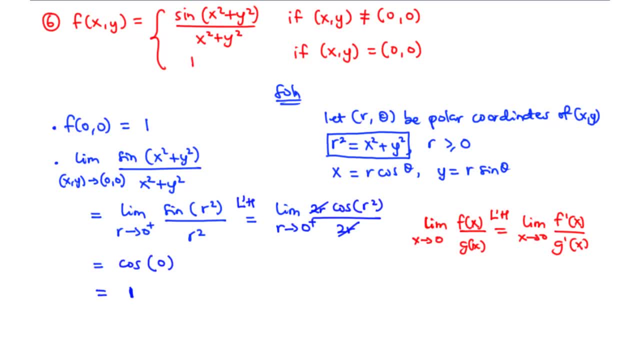 Whenever you obtain the limit of a function using the polar coordinate approach, It does not necessarily mean that the limit of the function is what you obtain. You will still need to use the precise definition of function, That is, the epsilon delta definition of limit. 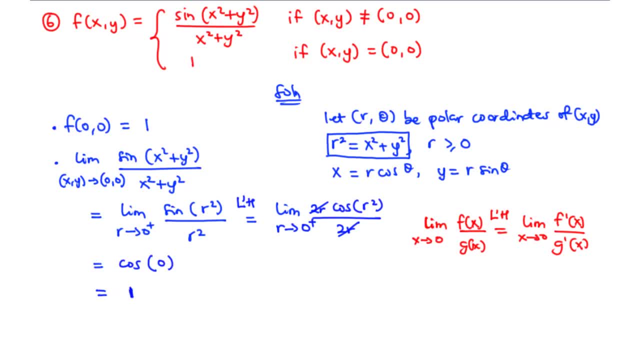 To prove that the value you had is actually correct. Now, the reason why we are using this approach For this particular question is that The actual limit of this function Is equal to the value we have here. The actual limit of this function is equal to the value that we have here. 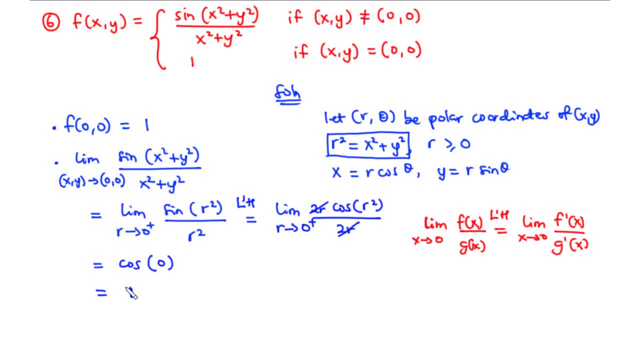 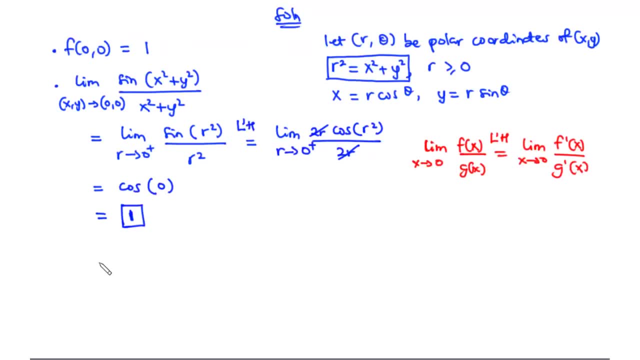 That is why we chose to use the polar coordinate approach. So the value of the limits of this function is equal to 1.. Therefore, Therefore, Since the limit of the function, The limit of the function f of x y, As x y approaches the point 0, 0.. 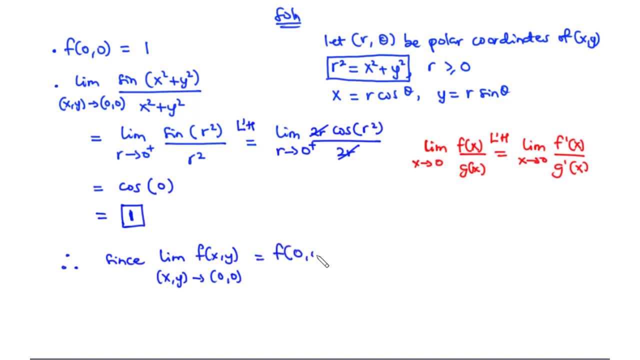 Is equal to the value of the limit at the point 0, 0.. We say that the function f of x, y Is continuous, Is continuous At the point 0, 0.. Now to the last question, Question 7, or example 7.. 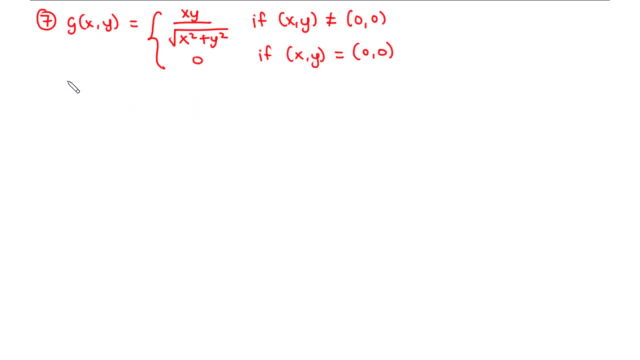 We have: g of x- y equals x- y over the square root of x squared plus y squared If x- y is not equal to 0, 0. And then 0 if x- y is equal to 0, 0.. 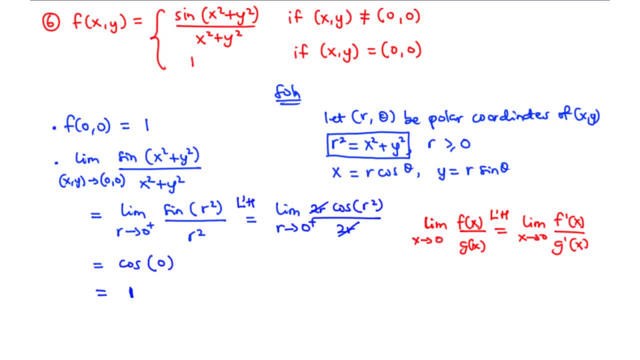 is equal to the value you obtain. whenever you obtain the limit of a function using the polar coordinate approach, it does not necessarily mean that the limit of the function is what you obtain. you will still need to use the precise definition of limit, that is, the epsilon delta definition of. 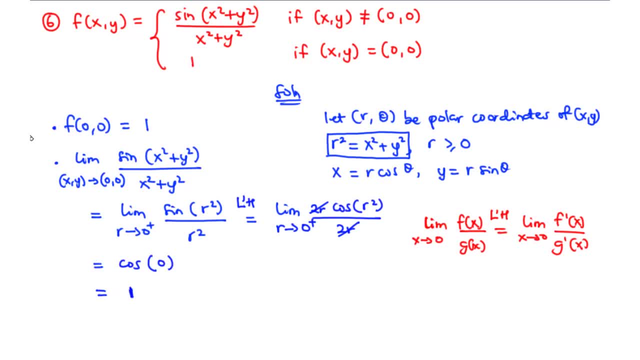 limit to prove that the limit of the function is equal to the value of the function. the value you had is actually correct now. the reason why we are using this approach for this particular question is that the actual limit of this function is equal to the value we have here. 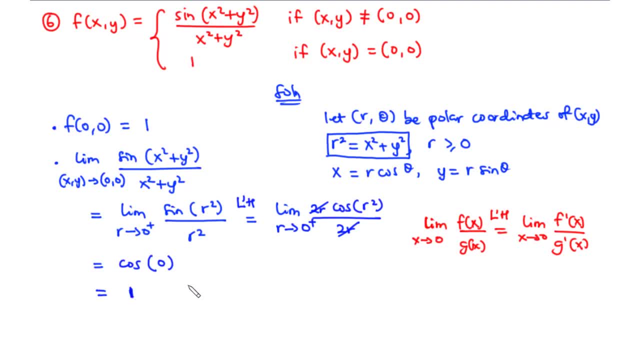 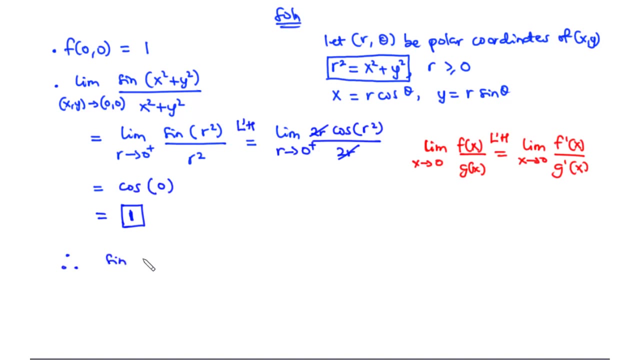 the actual limit of this function is equal to the value that we have here. that is why we chose to use the polar coordinate approach, so the value of the limits of this function is equal to 1. therefore, therefore, since the limit of the function, the limit of the function f, of f, of x, y, as x y approaches the point zero, zero. 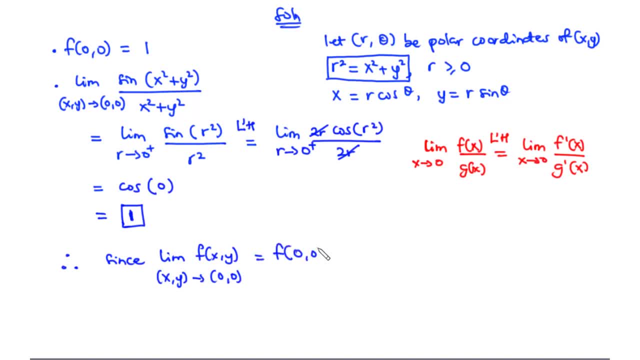 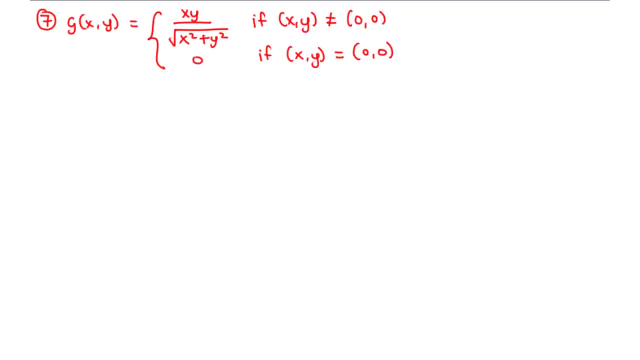 is equal to the value of the limit at the point zero zero. we say that the function f of x y is continuous, is continuous at the point zero zero. now to the last question, question seven, or example seven. we have: g of x- y equals x y over the. 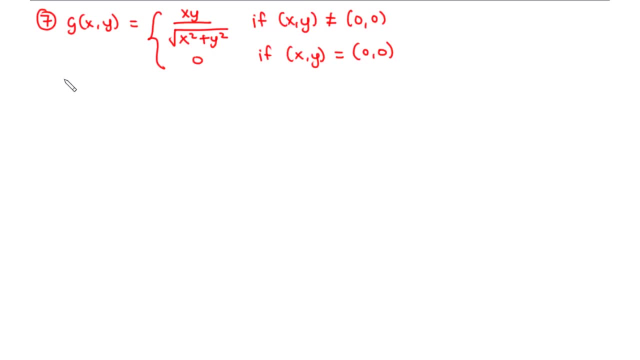 square root of x square plus y square. if x, y is not equal to zero, zero and then zero. if x, y is equal to zero, zero. now let's try this together. so, as usual, we first of all find g of zero, zero, and that is defined. that is equal to zero. secondly, 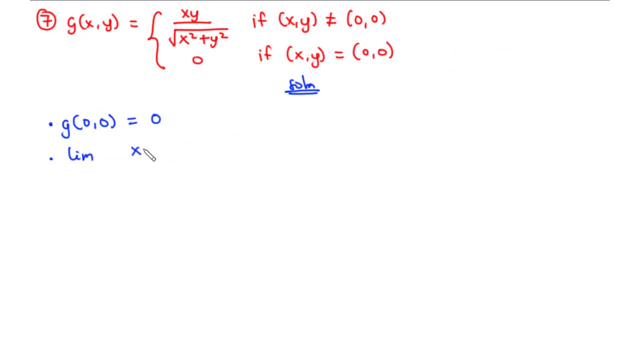 we want to find the limits of the function x- y over the square root of x square plus y square, as x y approaches zero zero. also, for this example, we are going to use polar coordinates. so we know that x is equal to r cos theta. we have y to be r sine theta and then r square equals x square plus. 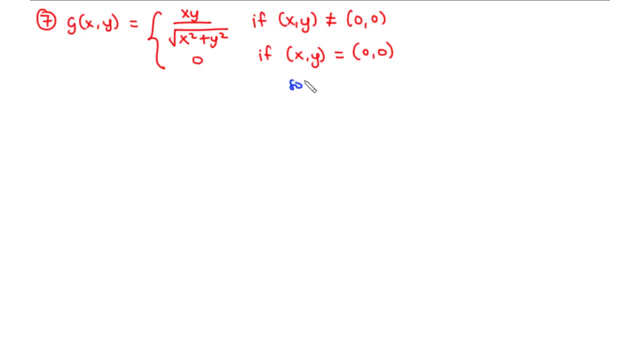 Now let's try This together. So, as usual, We first of all find G of 0, 0. And that is defined. That is equal to 0.. Secondly, We want to find the limits of the function x- y over the square root of x squared plus y squared. 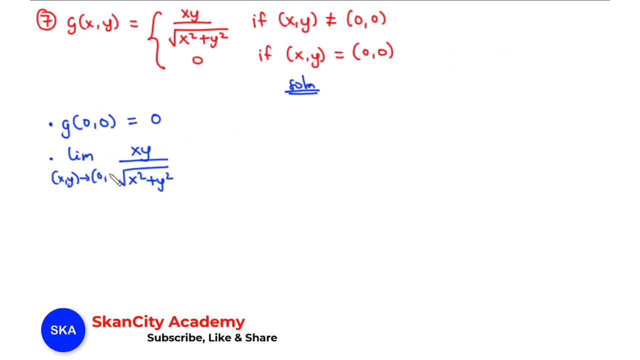 As x, y approaches 0, 0.. Also, for this example, we are going to use polar coordinates, So we know that x is equal to r cos theta. We have y to be r sine theta And then r square equals. 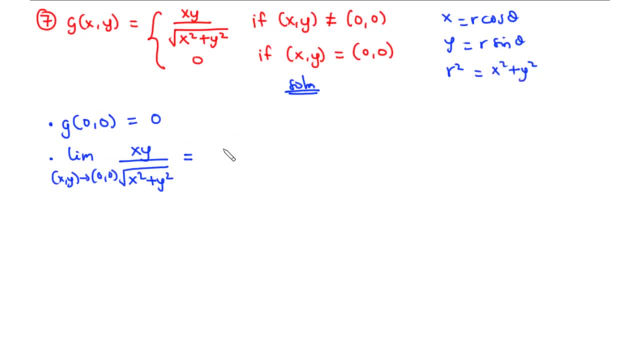 x squared plus y squared. So with this we are going to have the limits of the function. we have x To be r cos theta times y, which is r sine theta. So we multiply the two and then we have. 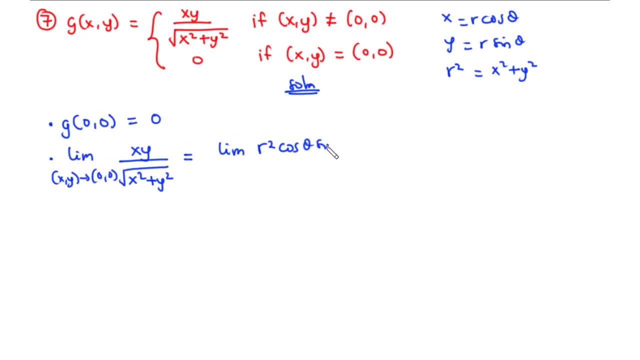 r squared cos theta sine theta, all divided by, And for the square root of x squared plus y squared, we basically Take the square root of both sides and then we have r to be equal to the square to of x squared. 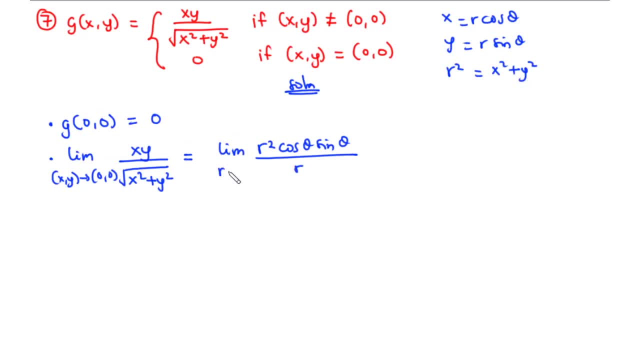 Plus y square. so this is basically r as r approaches zero from the right. this is equal to: we are going to cancel out this r and then one of the r's on top, so that we have the limit as r approaches zero from the right of r cos theta sine theta. at this point you can do direct substitution. 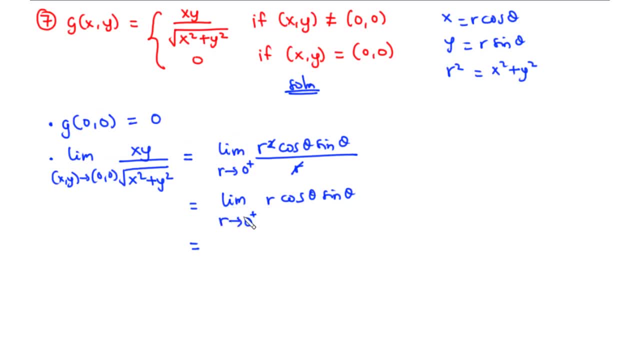 so that we substitute zero in place of r, so that we have zero, so we have zero times cos theta, times sine theta, and this is equal to zero. so the limit of the function, as x, y approaches zero, zero is equal to zero. and notice that this is the required limits of the function. 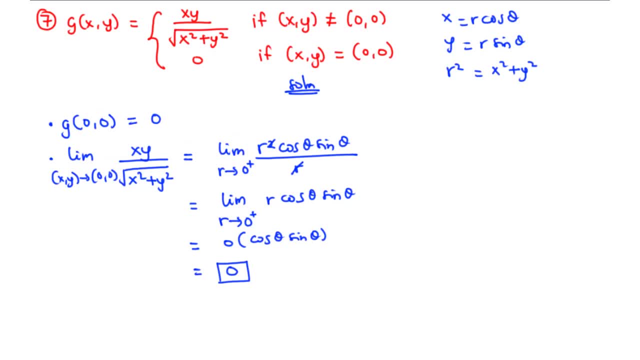 as i said earlier on, using polar coordinates to find the limit of a function that is equal to zero, so that we have zero, so we have zero. times cos theta, times sine theta does not guarantee that the value you obtain at the end is the limit or the required limit. 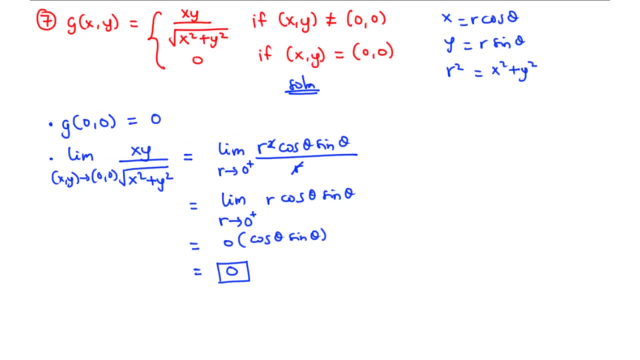 of the function. the reason why we used polar coordinates is just because, for this particular question or for this particular function, the limit we obtain, or the value we obtain, is the actual limit of the function. so we have the limit of this function as x, y approaches zero, zero to. 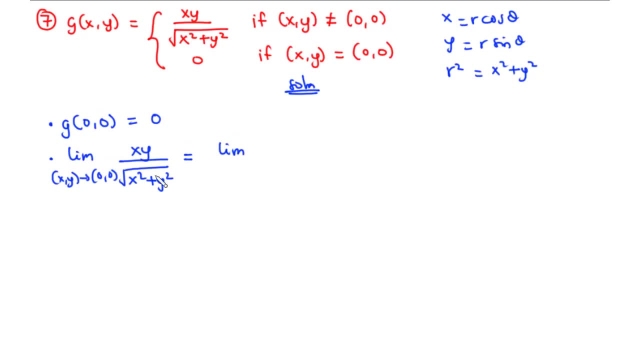 y square. So with this we are going to have the limit of the function. We have x to be r cos theta times y, which is r sine theta. So we multiply the two and then we have r square cos theta sine theta, all divided by, and for the square root of x square plus y square, we basically 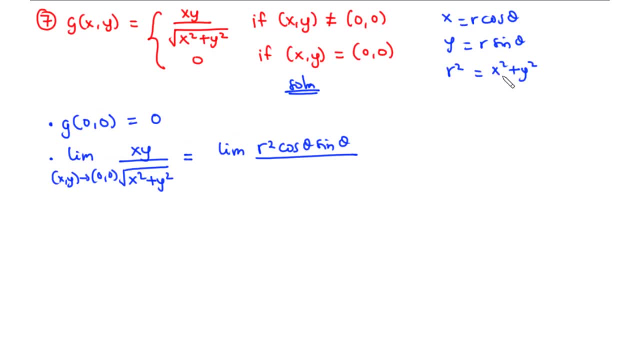 take the square root of both sides and then we have r to be equal to the square root of x square plus y square. So this is basically r. as r approaches zero from the right, this is equal to: we are going to cancel out this r and then one of the r's on top so that we have the limit. 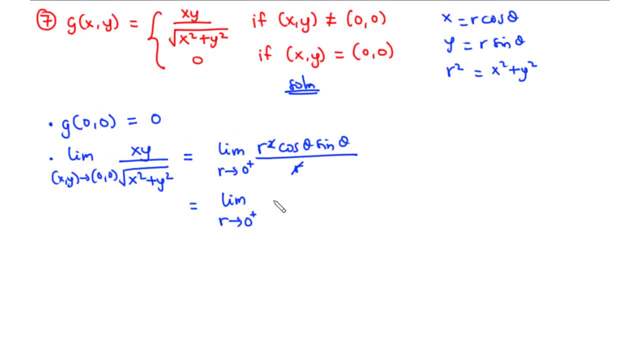 as r approaches zero from the right of r: cos theta sine theta. At this point you can do direct substitution, so that we substitute zero in place of r, so that we have zero. So we have zero times cos theta, times sine theta, and this is equal to zero. 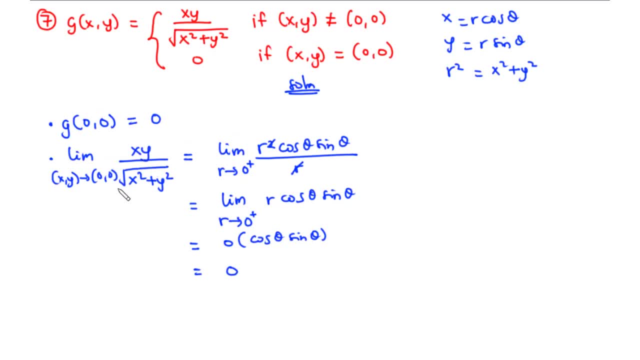 So the limit of the function as x, y approaches zero. zero is equal to zero, and notice that this is the required limits of the function. As I said earlier on, using polar coordinates to find the limit of a function does not guarantee that the value you obtain at the end is the limit, or 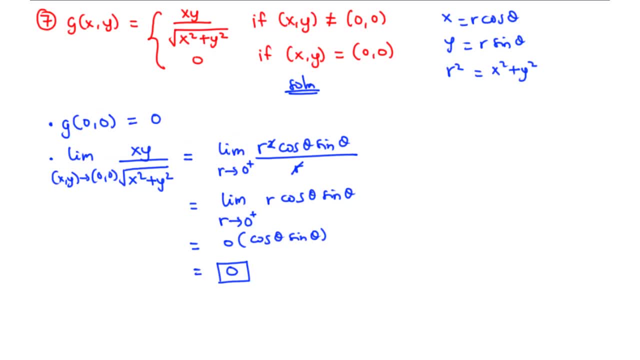 required limit of the function. The reason why we used polar coordinates is just because for this particular question or for this particular function, the limit we obtain, or the value we obtain, is the actual limit of the function. So we have the limit of this function as x, y approaches 0,, 0 to be. 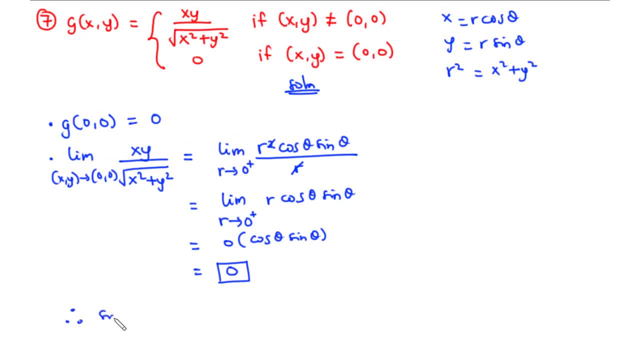 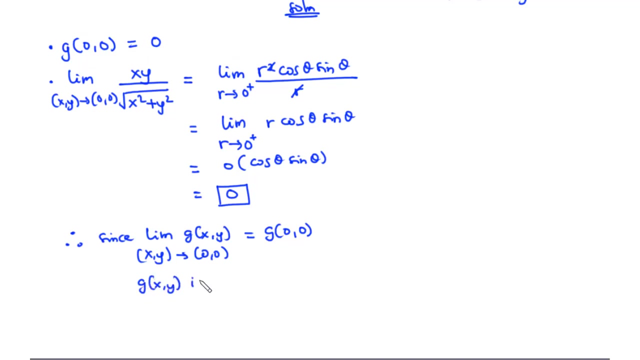 equal to 0.. Therefore, since the limit of the function g of x- y, as x y approaches 0,, 0 is equal to the value of the function at point 0, 0,, we say that g of x- y is continuous. This is: 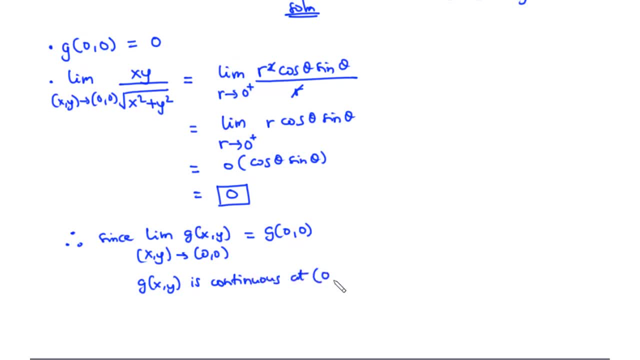 continuous at point 0, 0.. That's the point 0, 0..